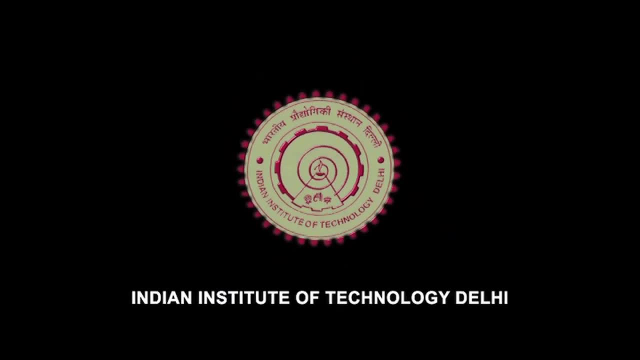 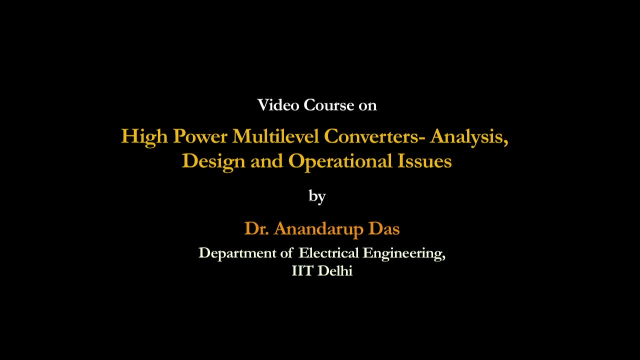 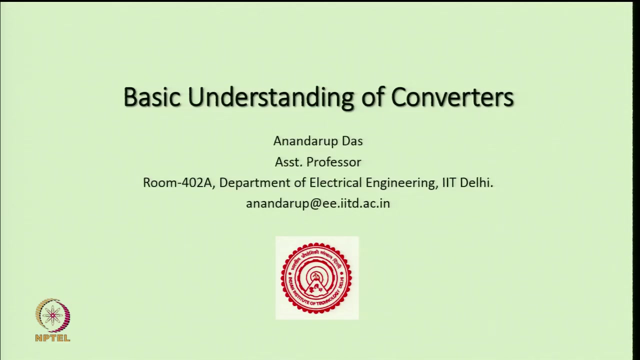 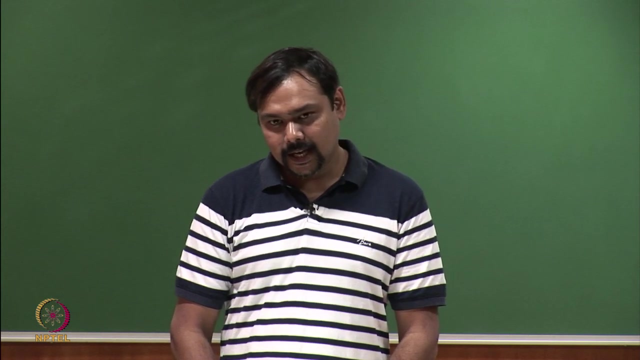 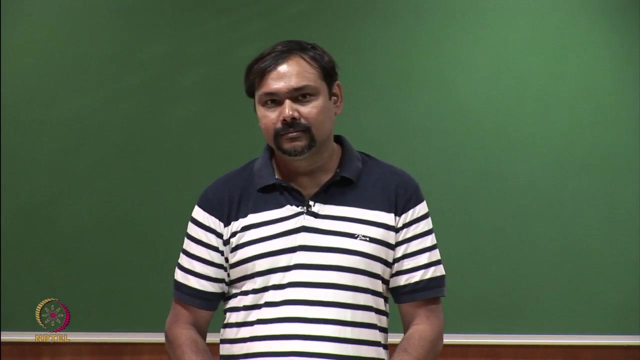 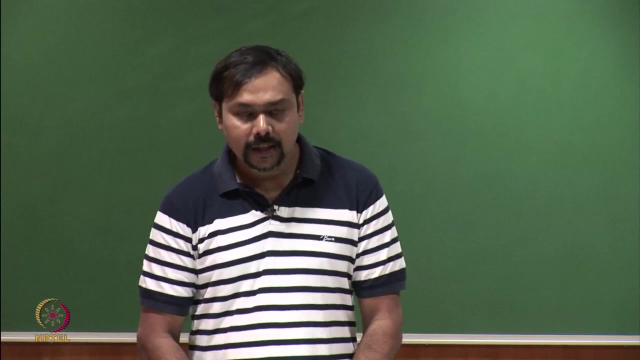 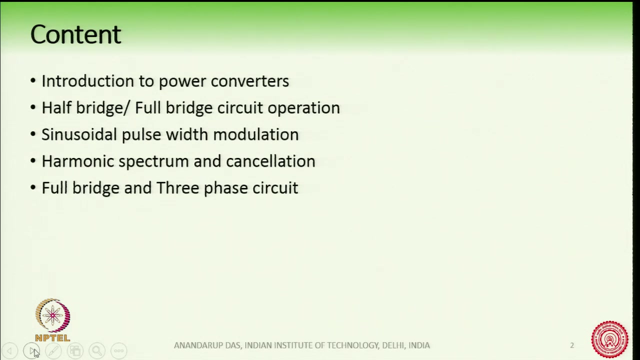 So we start with the first lecture of this course and which is basic understanding of converters. So in this one, in this section, we will cover the basic introduction to power converters. we will study half bridge, full bridge, circuit operation, little bit about sinusoidal pulse width modulation, and then full bridge and 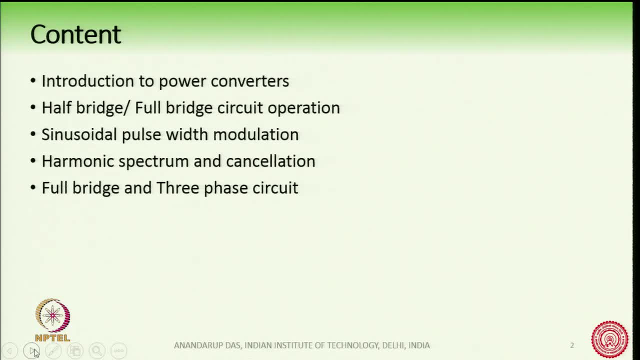 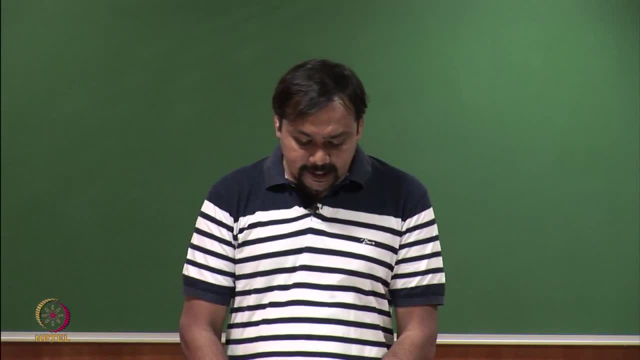 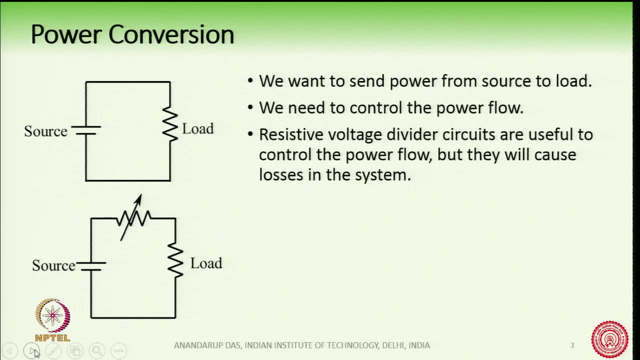 three phase circuits. So the basic power conversion. when we talk about power conversion, of course we talk about a source of energy and a sink of energy, or we have a source and a load, So we want to send the power from the source to the load. So here you can see that we have a power. 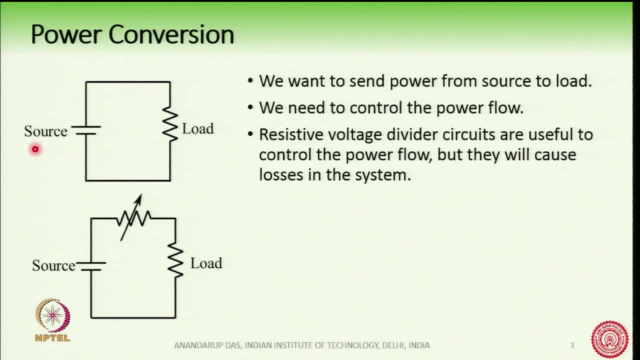 conversion. we have a source here and we have a load here. We are assuming the load to be a resistive load here. So if we connect or if we analyze this circuit, this is a DC source and a load. we see that energy is flowing from the source to the load, but there is 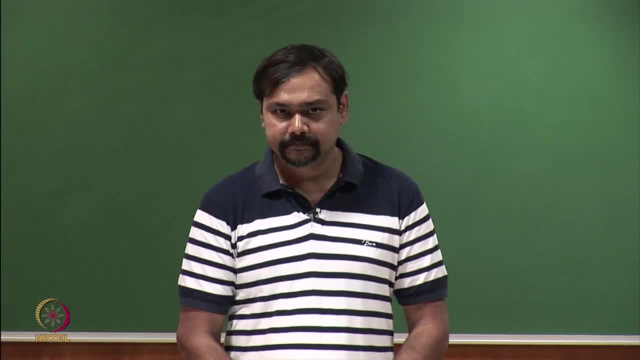 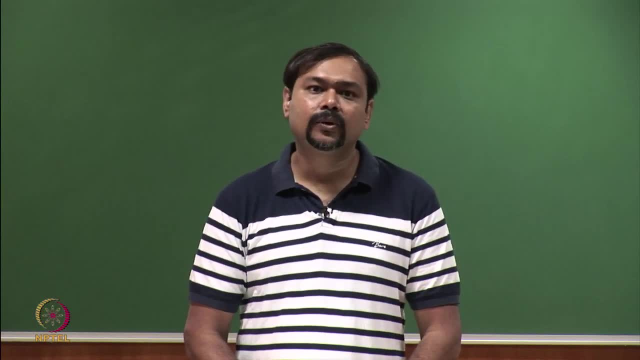 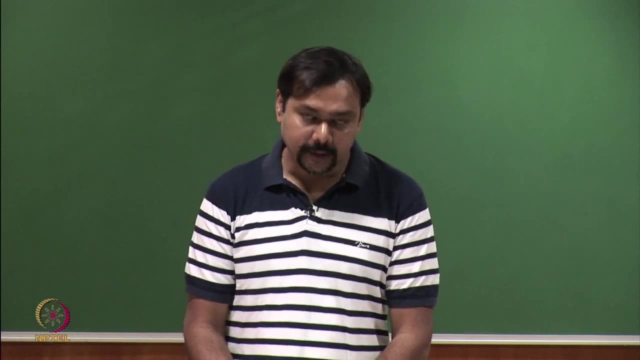 no control of the flow of energy. ok, So it is a fixed source and a fixed load and we cannot control the flow of power from the source to the load. So how can we control the power flow? The easiest way of doing it is to add a potential. 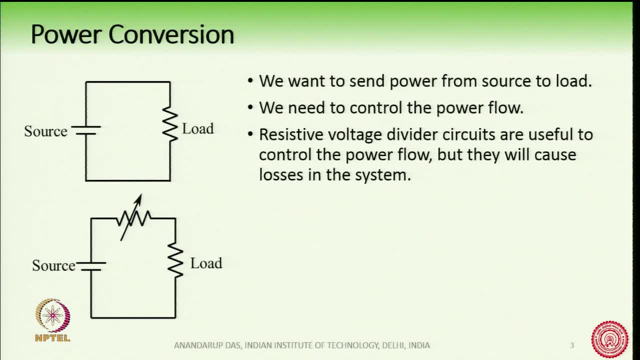 divider, a resistive voltage divider, as it is shown in the slide, And this is the easy colour weght of determineing the loss distance which we would attach to the specific component joint. And so we areaintiding this frequency, and what will you do about the resistance fate? 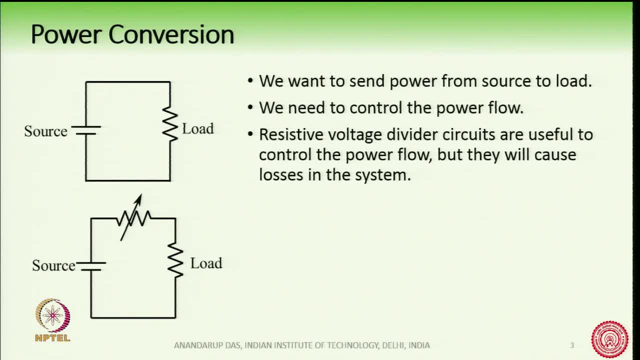 as the Rayleigh стал ordered local from the source. Well to few fill the thickness more clear Answers to quick question. you may have the following proof in order: the control command, 2nd figure: the resistive voltage divider. here Now, if I add the resistive voltage divider, 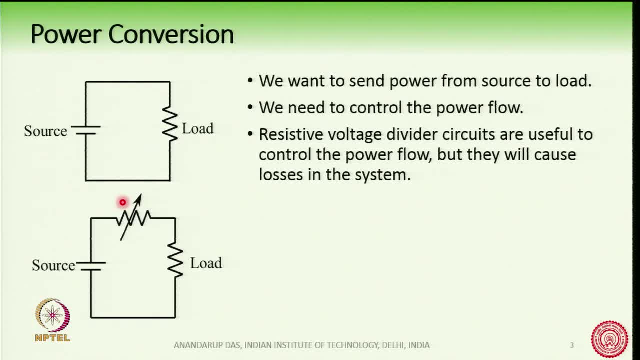 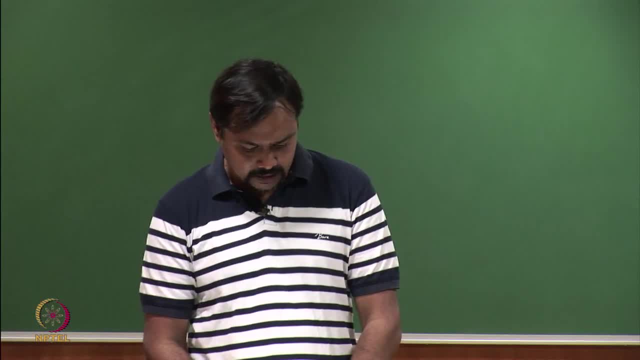 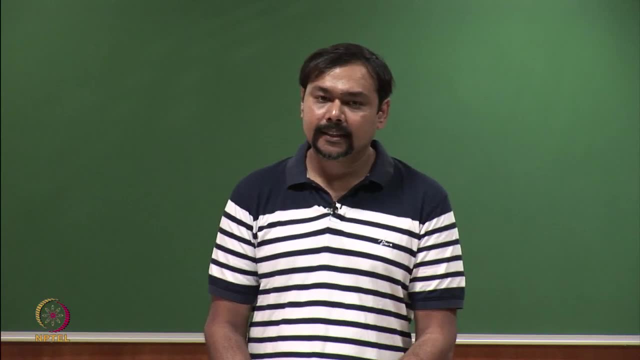 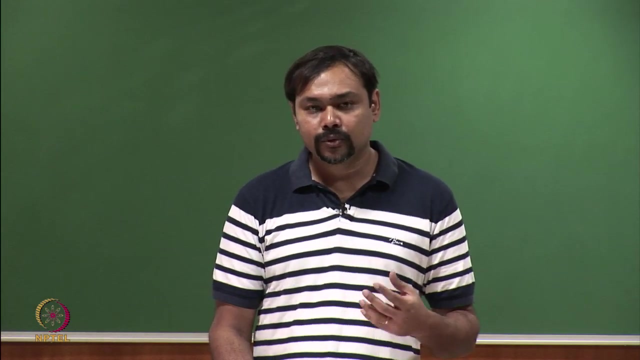 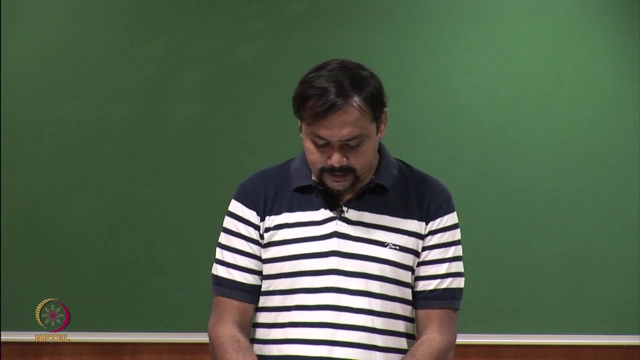 and by varying this resistance on the variable resistance, I can control the flow of power into the load. However, although this system will function, however, this is not an efficient system because when we transfer the power through the voltage divider or through the potential divider, or through this resistive voltage divider circuit, we lose a substantial 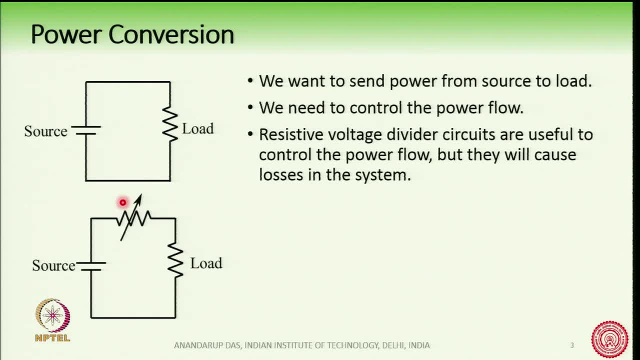 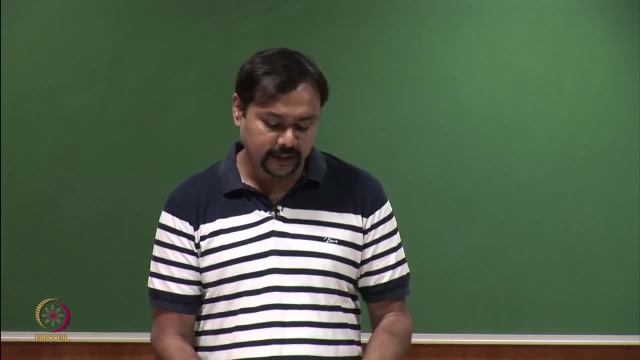 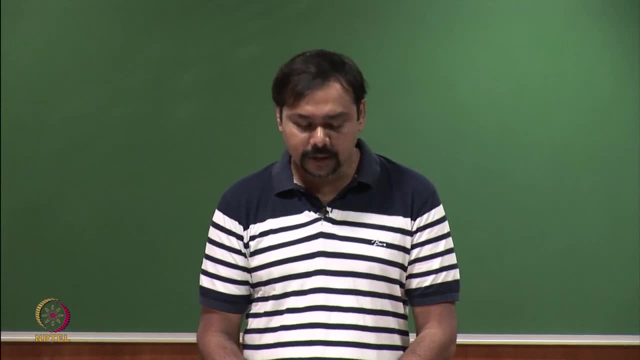 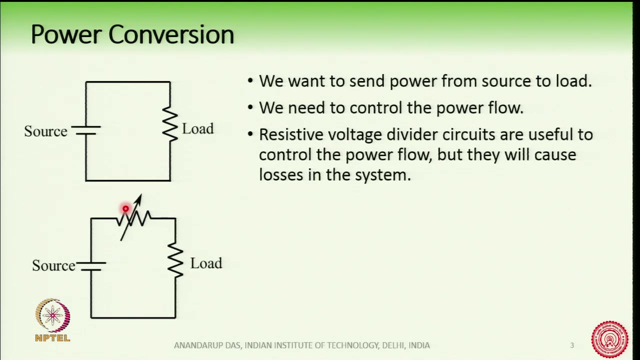 amount of power. So, in particular when we talk about high power levels, is not at all suitable. this circuit is not at all suitable because it will cause a large amount of heat dissipation in this particular resistive voltage divider circuit and subsequently the efficiency of. 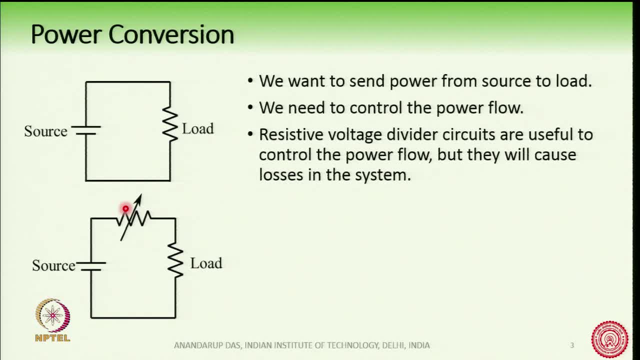 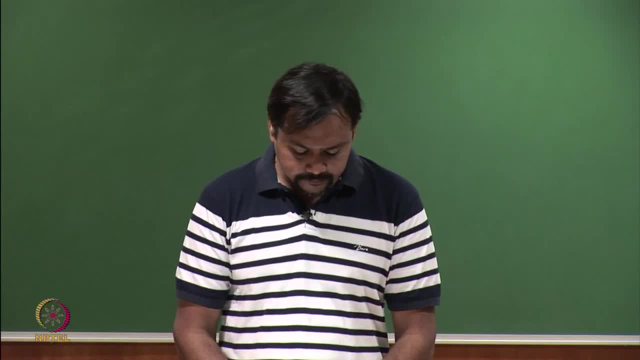 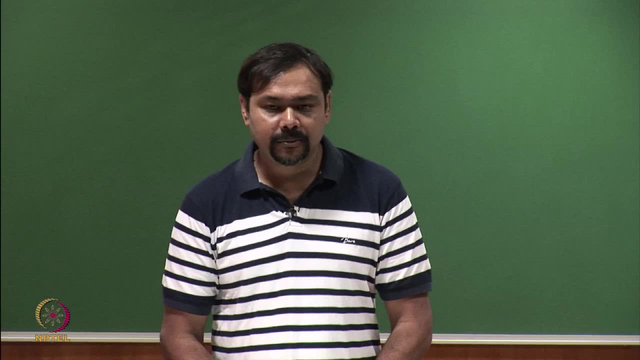 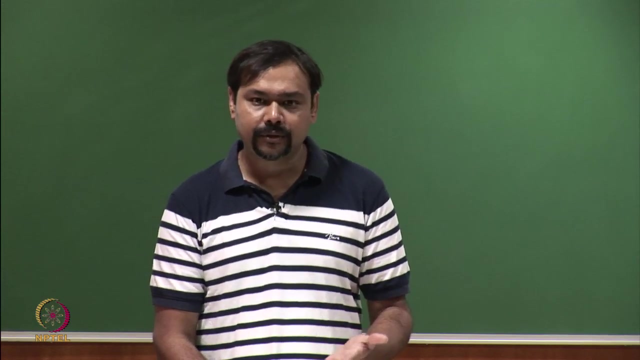 the system will go down. In all these high power converters, high power conversion efficiency is a very important factor and there are two reasons for that. The first reason why the efficiency is important is if you do not have the high efficiency, you lose the energy. So that is one important factor for any system that you want to, whatever. 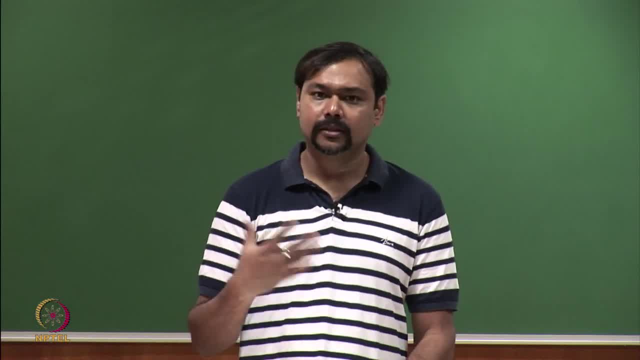 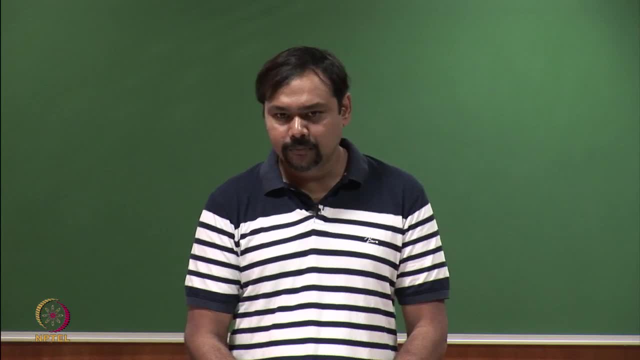 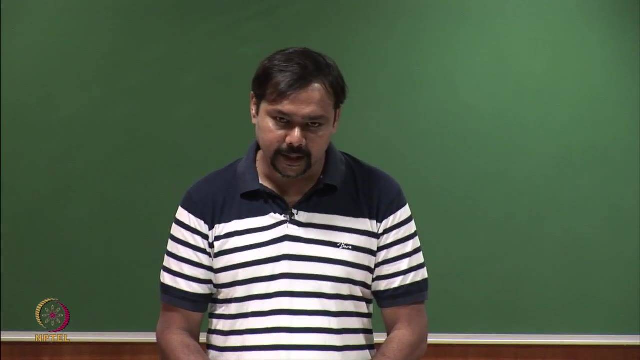 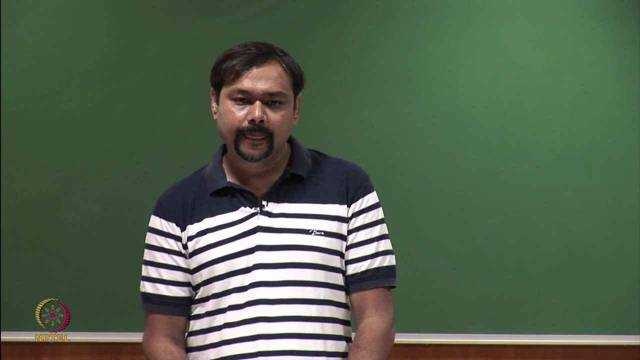 is the desirable power flow. you want to do it with the maximum efficiency. So this is, you get the maximum energy from the input. But there is another very important reason why efficiency should be very high, because if efficiency is not high, then the losses. 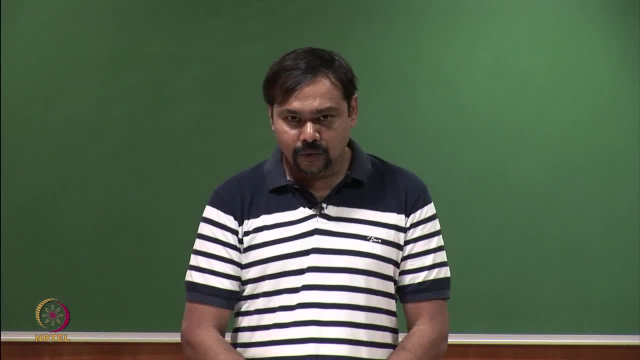 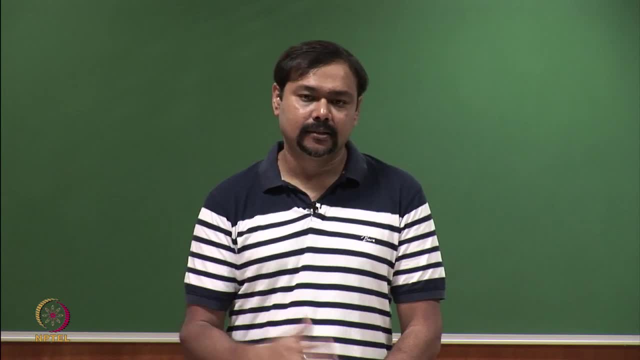 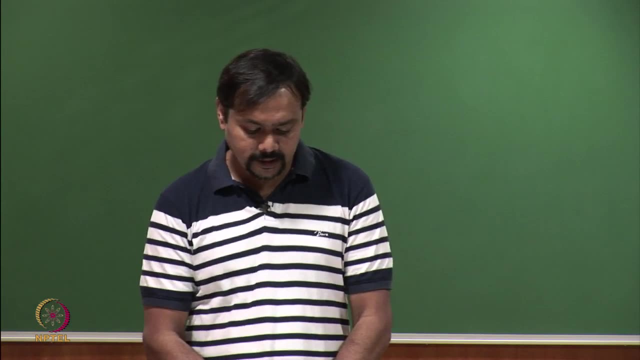 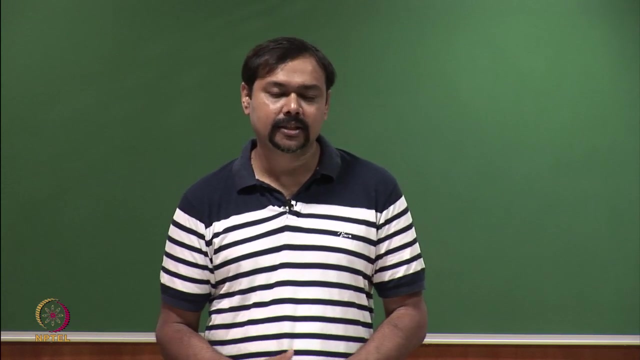 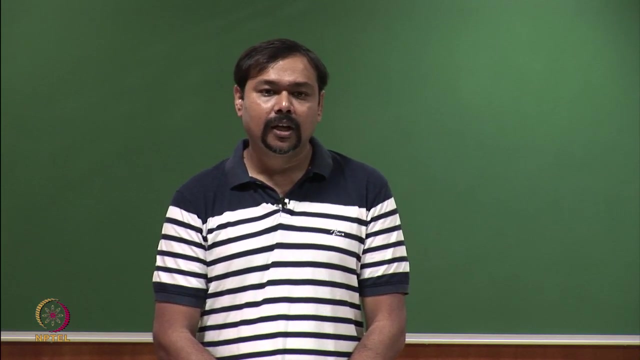 in the system is very high. So if the loss in the system is very high then it appears as heat in the system which we need to dissipate. You must have seen power converters with heat sinks, typically aluminum heat sinks. it is very frequently we have seen Heat sinks constitute 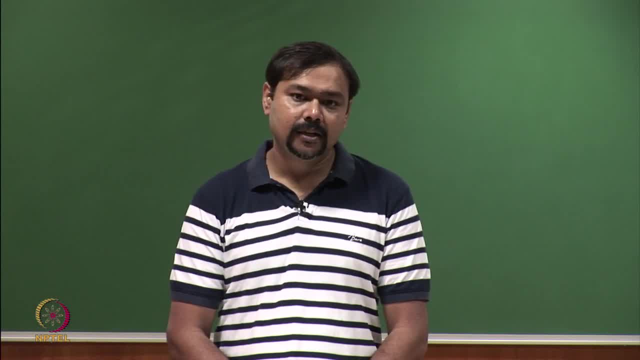 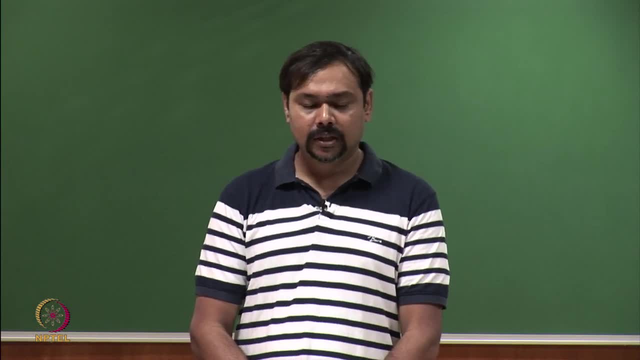 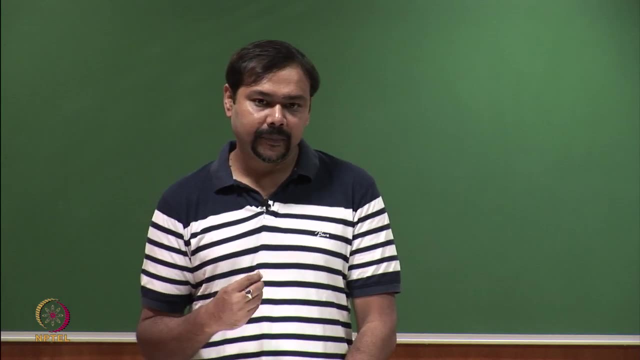 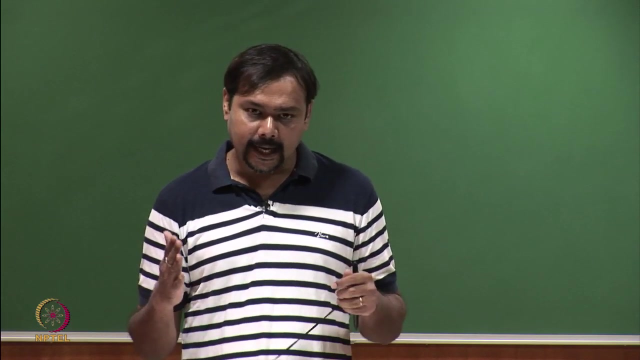 a major component in all power converters because it occupies a substantial volume and also a weight of the converter. So if the efficiency is low, that means the losses in the system is high, which in turn means that the high size of the heat sink should be bigger. 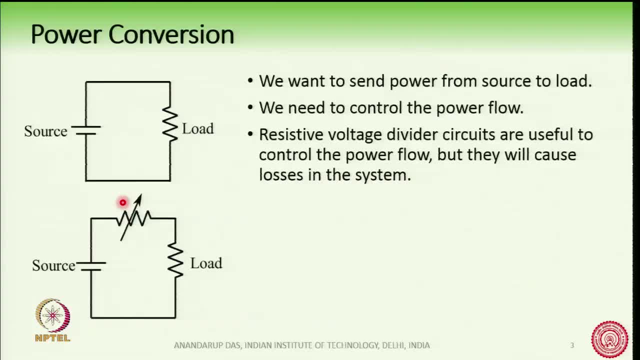 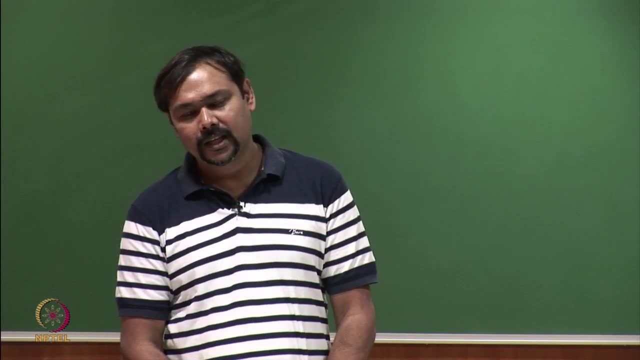 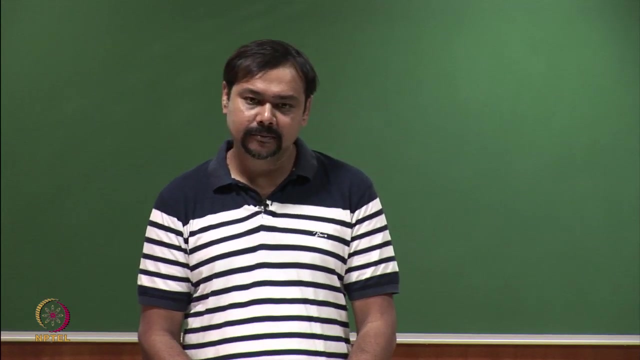 because we have to get the heat out of the system. So let us take the example of power converter, which is Handling about 1 megawatt of power. Suppose there are two converters and the first converter runs at an efficiency of 99 percent and the second converter runs at an efficiency of 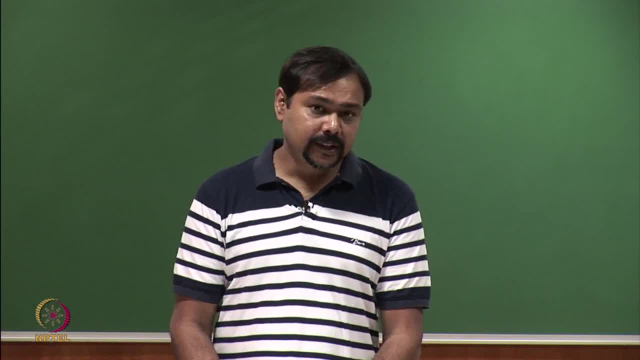 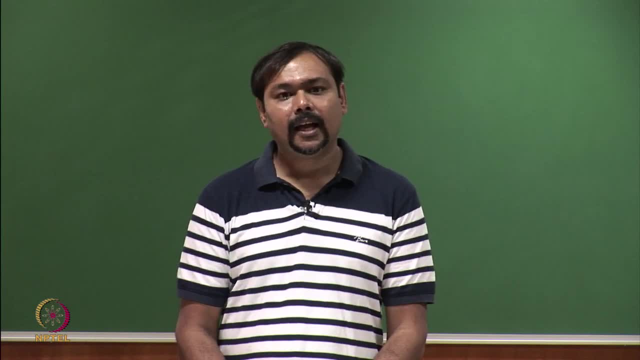 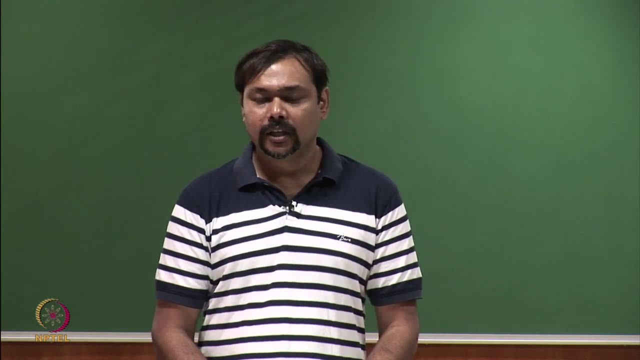 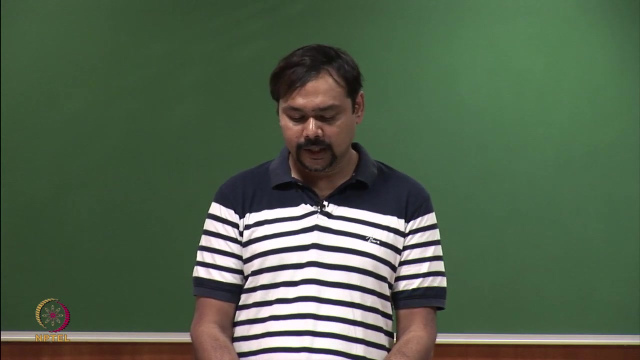 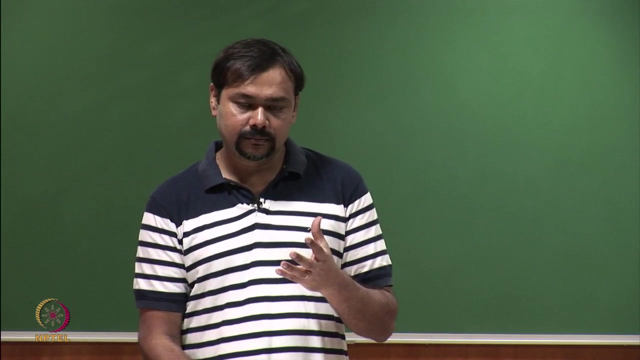 95 percent. Now. in the first converter the losses in the system is 1 percent of 1 megawatt And which is equal to 10 kilowatt, and for the second converter the losses are 5 percent, So the loss is equal to 50 kilowatt. Now this means that all this loss is appearing. 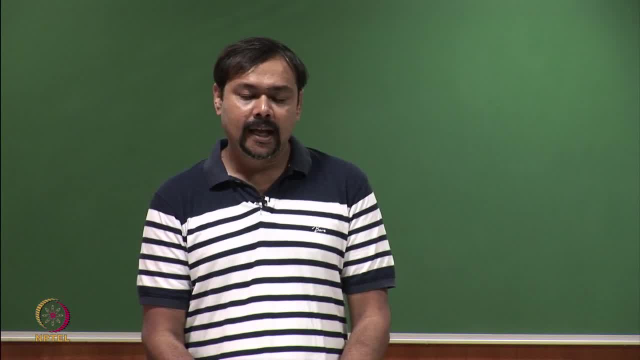 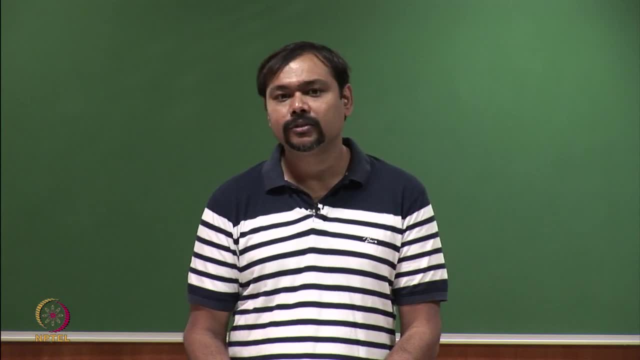 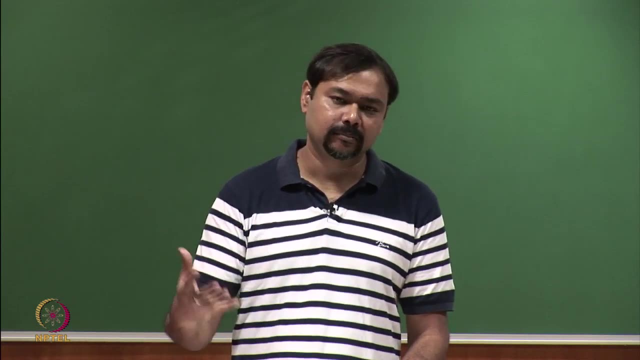 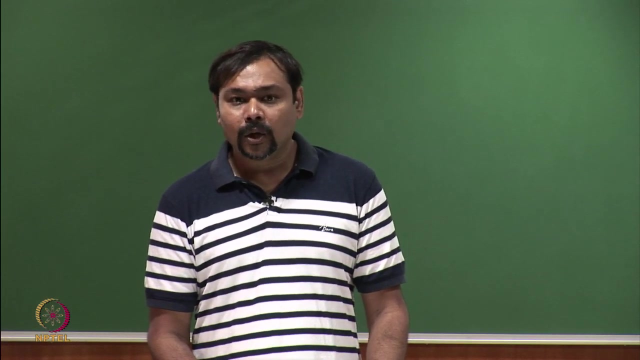 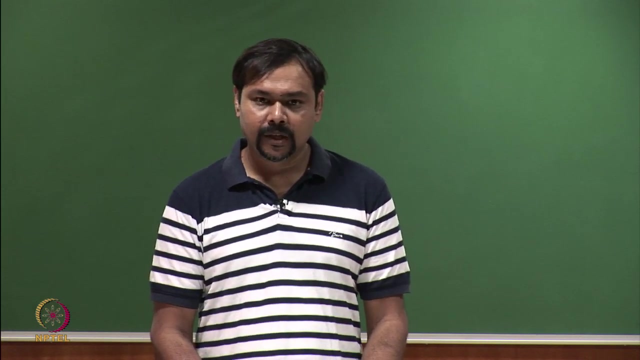 as heat in the power converter And which must be Total, totally dissipated into the ambient, either through by natural cooling by air, or by forced cooling through water or some kind of oil, for example. So the losses play a very vital role in the power conversion process and there is also 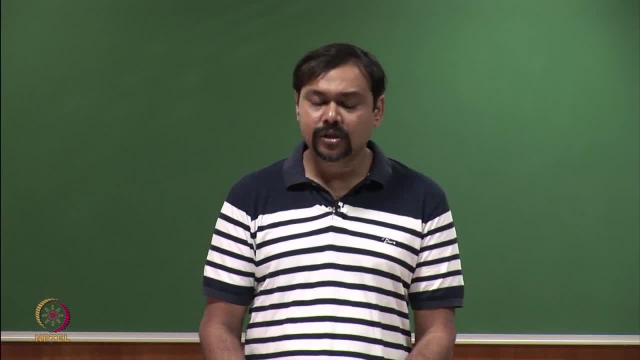 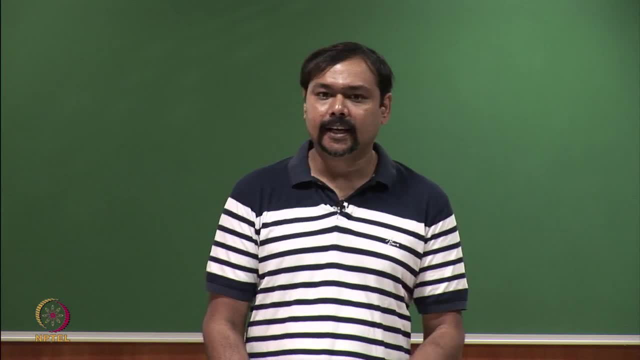 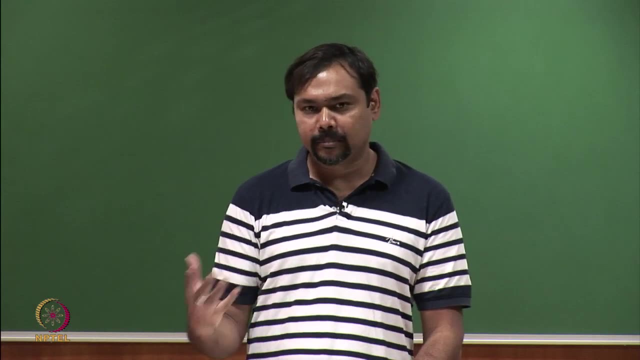 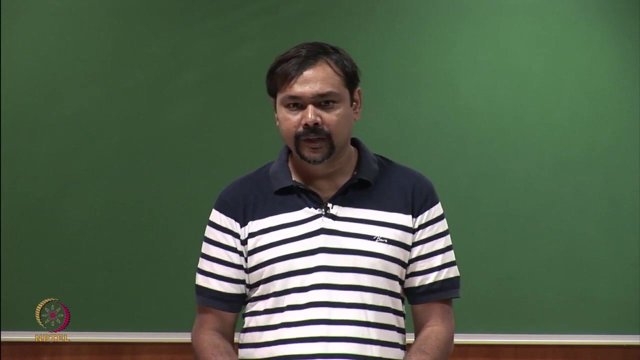 one principle which is usually followed in the industry. It says this is the Arrhenius principle, and it says that every 10 degree centigrade rise in the temperature of, say, a power device will reduce its lifetime by half. This is very important because if you operate a power device at an elevated temperature, 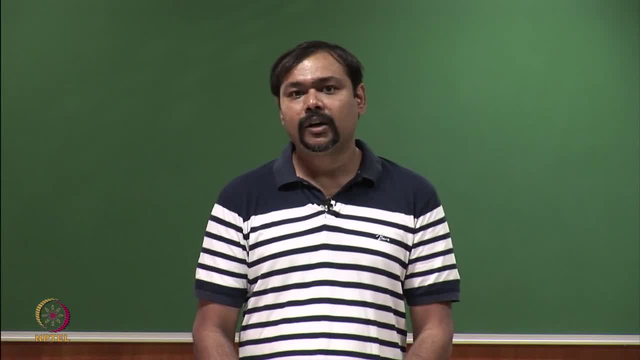 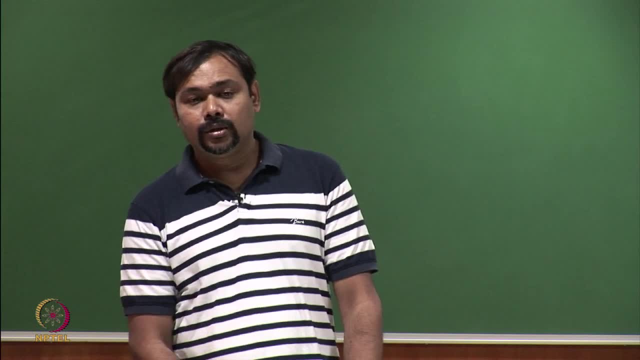 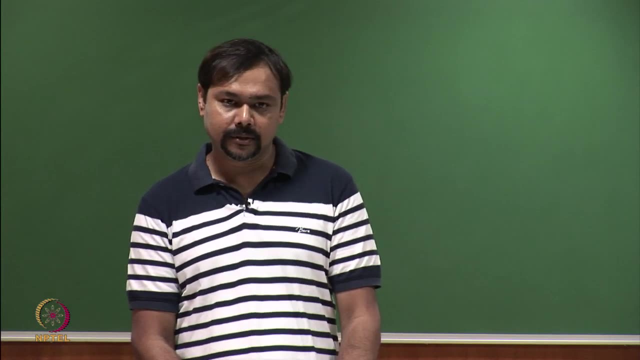 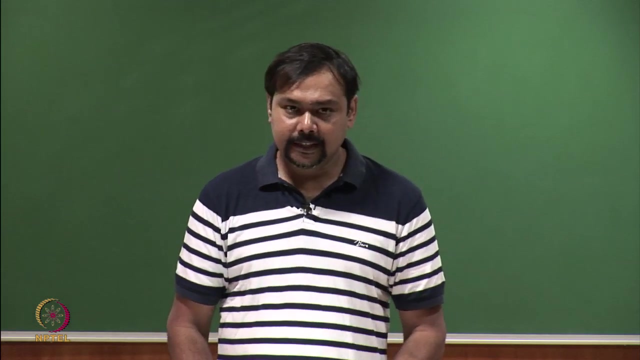 for prolonged duration of time, you are reducing the lifetime of the converter. So keeping the temperature under control in power devices or power converters is very important and there are lot of techniques to do that. Coming back to what we were discussing, so here we see that we have a source and we have 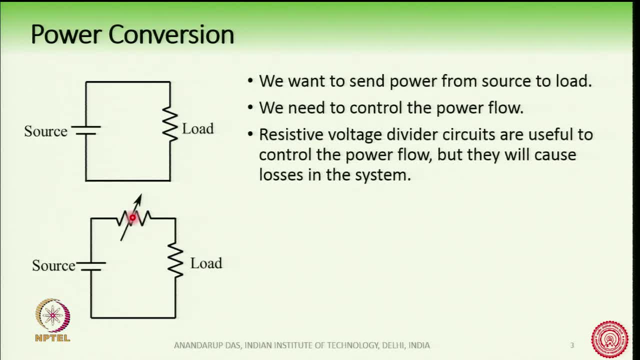 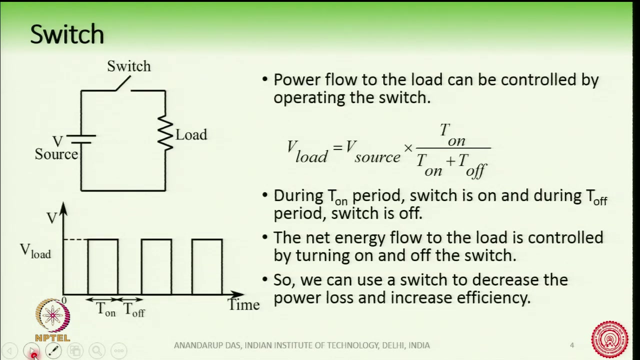 a load And the circuit, although there is a potential divider or a resistive voltage divider. but unfortunately this is not a very efficient circuit because a lot of heat will be dissipated in the potential divider. So we use so what is the solution for this? 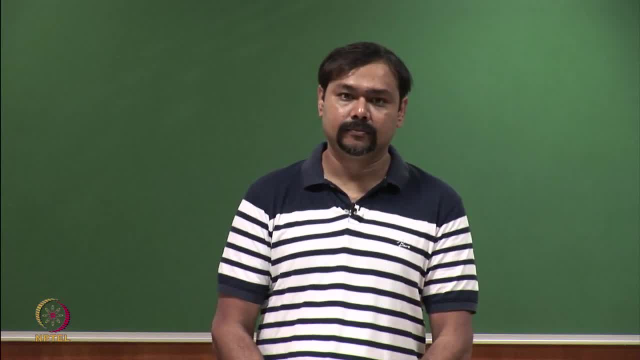 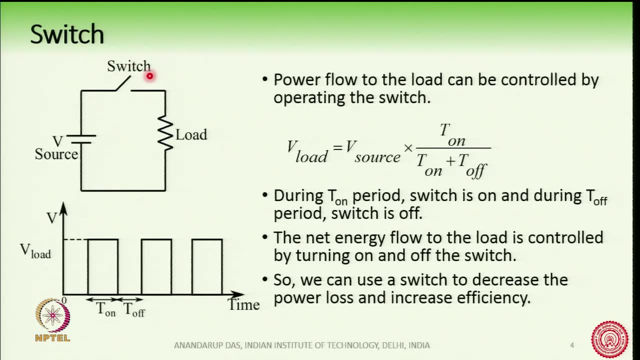 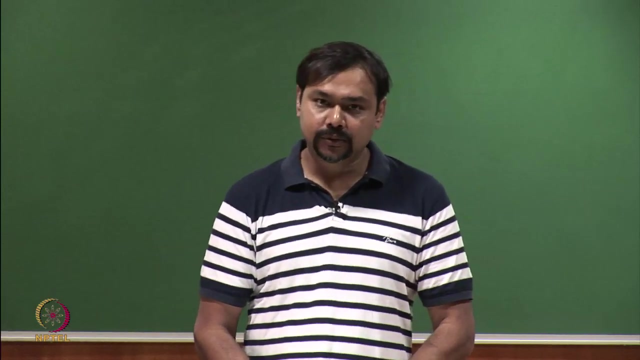 The solution for this is to use To use a switch which I have shown here. this is the switch here. Now, when you connect the switch, then suppose this is an ideal switch- I mean, it does not dissipate any heat, So- and it is a fully controllable switch, which means I can turn it on and I can turn. 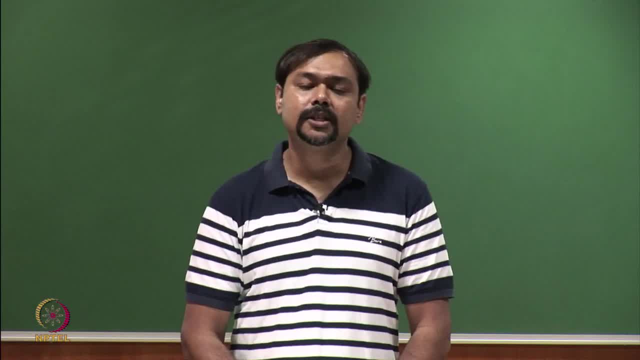 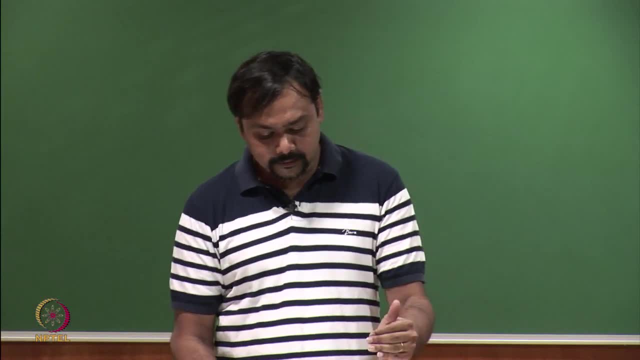 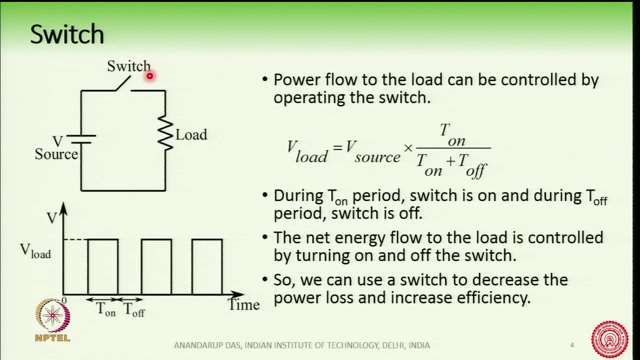 it off with control signals. So I can turn it off with control signals, which is totally controlled by myself or by me. So then we see that with this switch, power flow to the load can be controlled by turning on and off this switch. 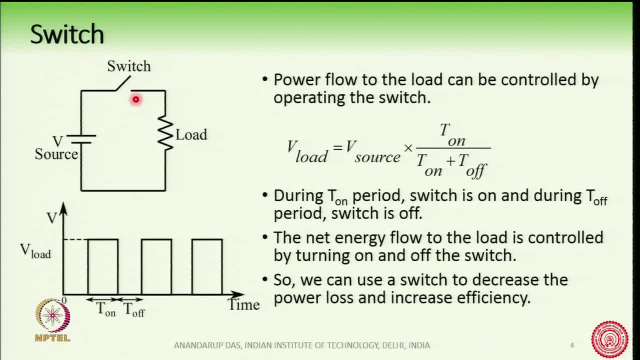 If I turn on the switch. if I turn on the switch, then the voltage of the source is impressed across the load. If I turn off the switch, no voltage comes across the load. So the voltage on the load is a series of pulses which is shown in this diagram. 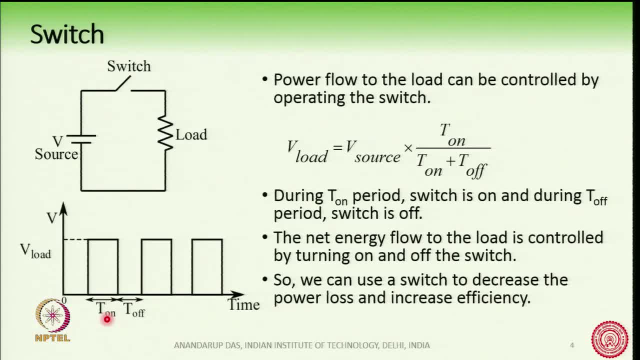 So when I turn on the switch, that is this t on period, then the load voltage is equal to the source voltage. When I turn off the switch, the load voltage is 0. So by controlling so, therefore, therefore, this V load which I have shown here, the expression: 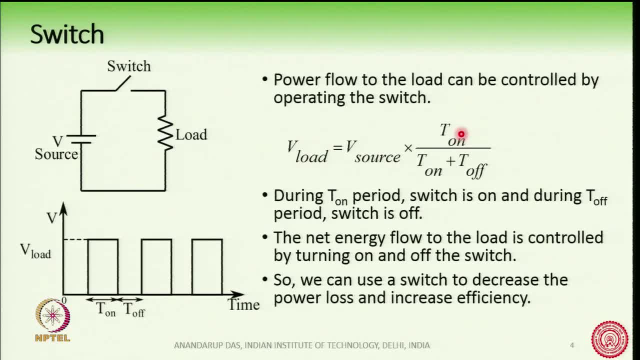 of V load is V source into t on, divided by t on plus t off, in an average sense. So therefore we see that the load voltage can be changed by changing the duration of t on over t off. So next question: Pulse voltage. it has an. 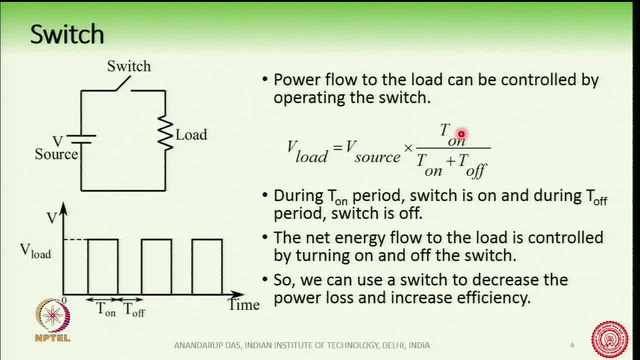 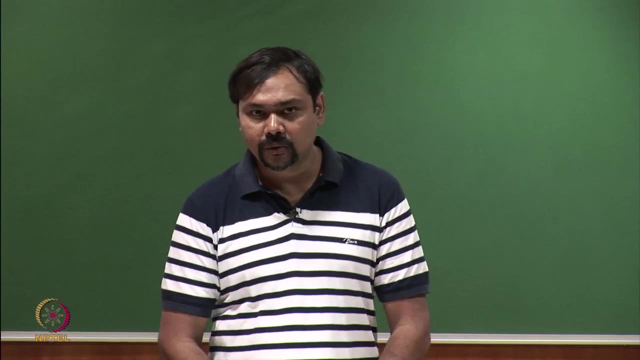 over this t on plus t off time. t on plus t off time is sometimes called the switching period. So we can change the magnitude of the load voltage, So we can use a switch to decrease the losses and increase the efficiency of power conversion from the source to the. 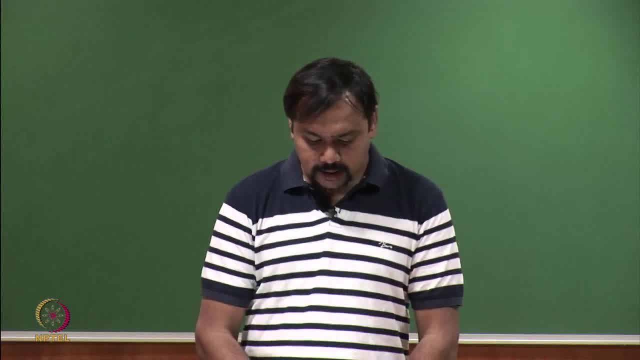 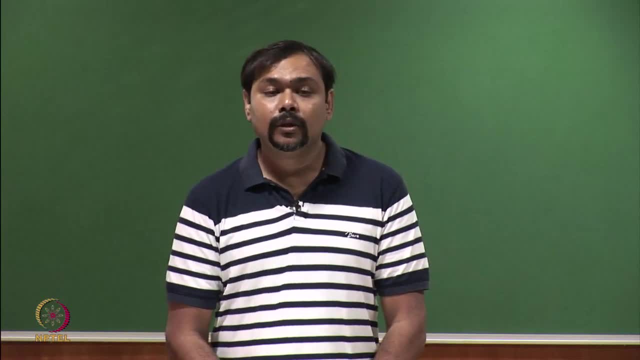 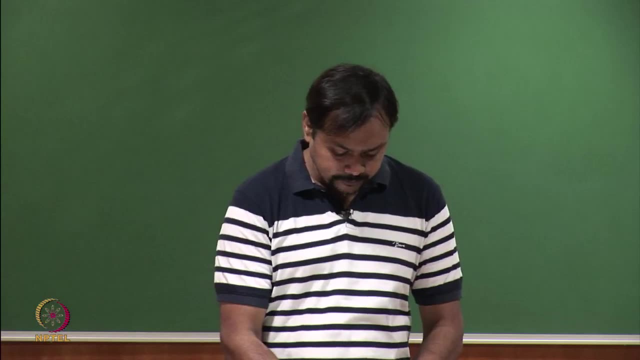 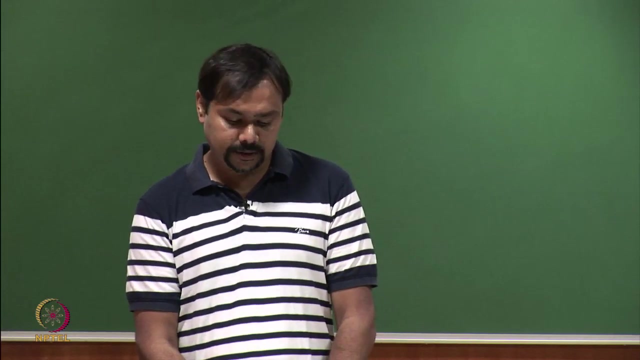 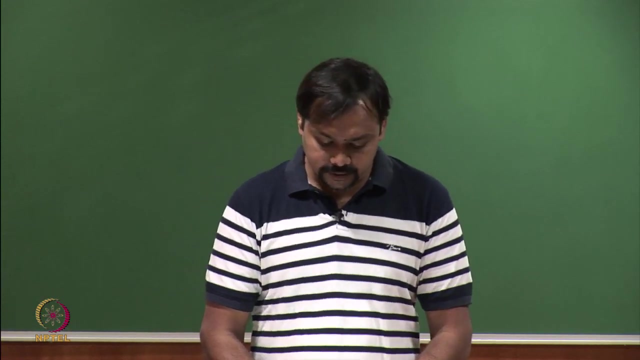 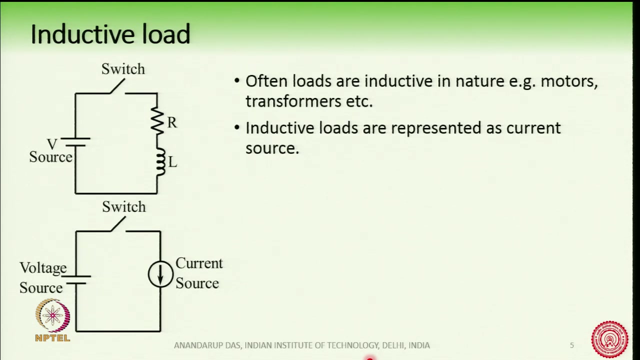 load. Now, although this arrangement of load and source with this switch works well for resistive loads, unfortunately most of the power electronic converters have inductive loads, that is, RL loads, resistive inductive load, or very poor, purely inductive loads or highly inductive loads. So often power electronic converters 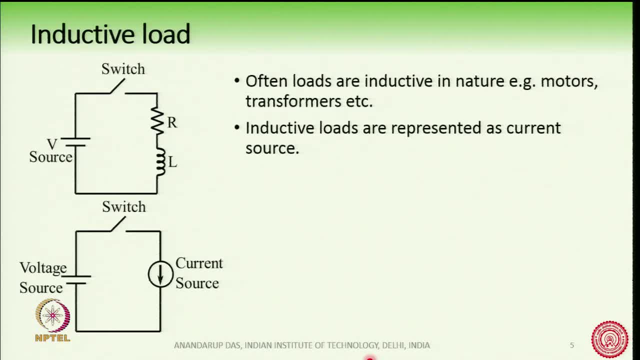 feed to loads, for example motors, transformers, etcetera. they are inductive in nature. Now, once the load becomes inductive in nature, we face a challenge, and that challenge is because of the property of inductive loads. Inductive loads are represented as current sources in the circuit. Now, current source: 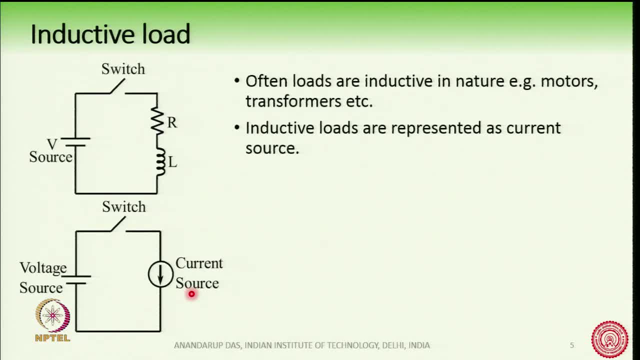 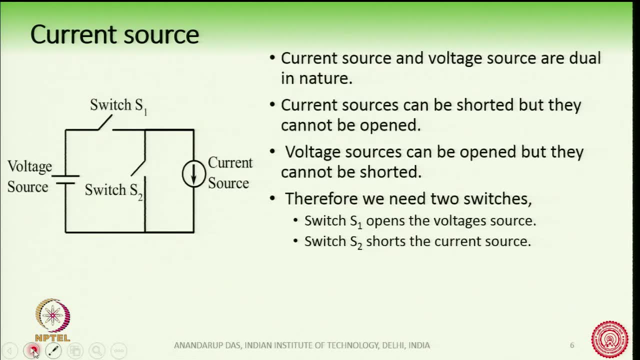 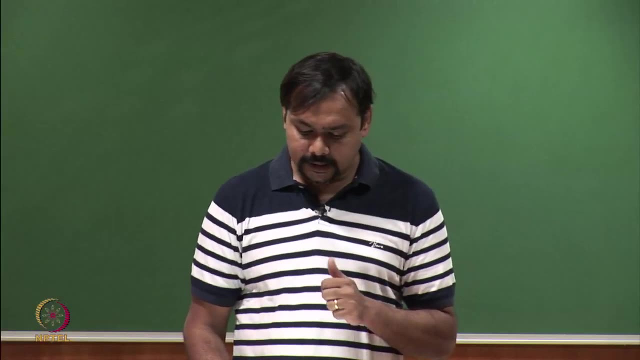 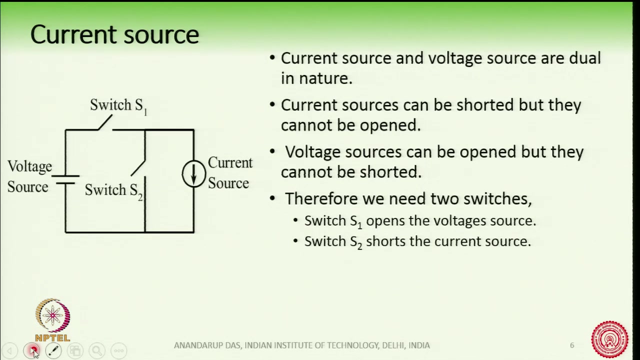 when you put into such a circuit along with a switch, then we face a challenge. What is the challenge? The challenge comes from the property of current source. You know current source and voltage source. they are dual in nature in terms of their properties. For example, current sources can be shorted, but they cannot be opened On. 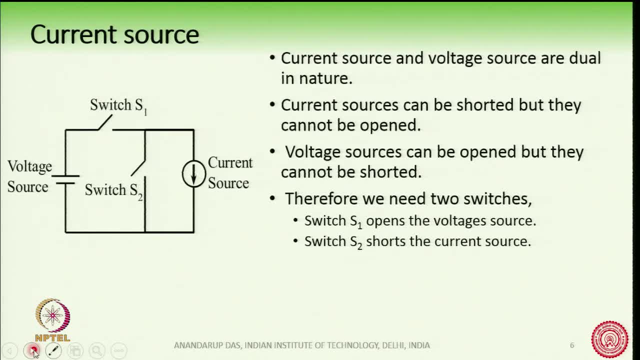 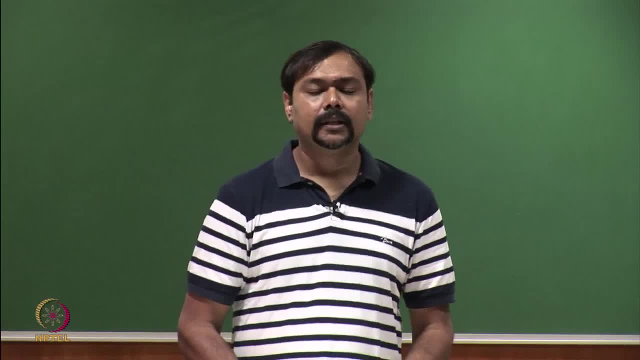 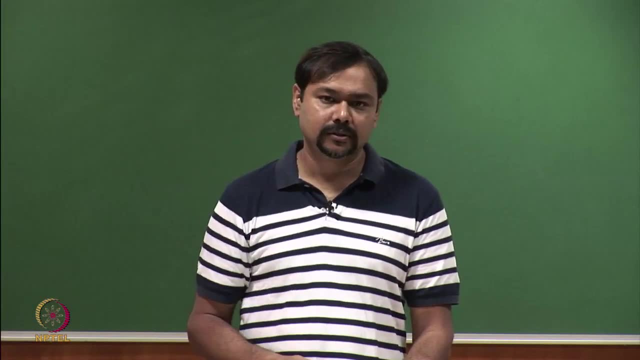 the other hand, voltage sources can be opened, but they cannot be shorted. For example, if you take a voltage source, say a battery, and then you can keep it open, You can take the volt battery in your hand and move round, nothing will happen because 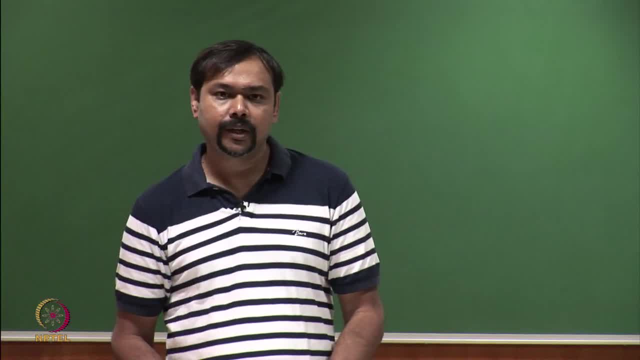 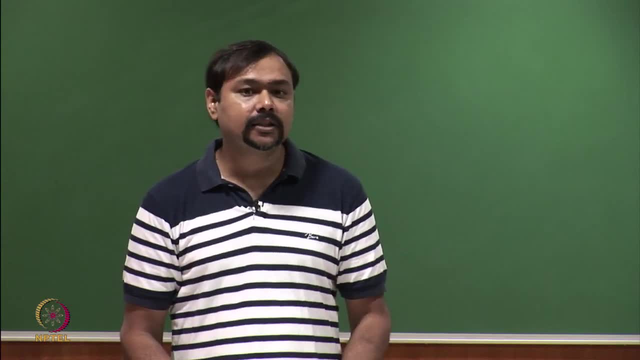 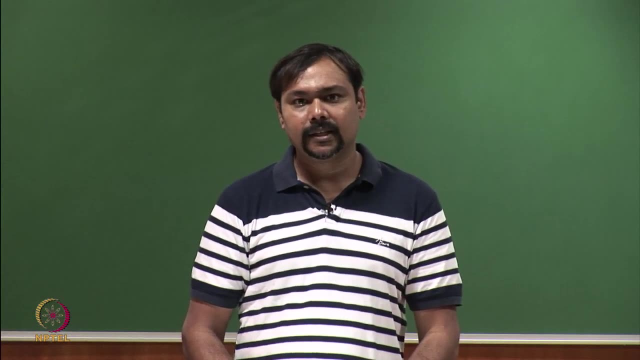 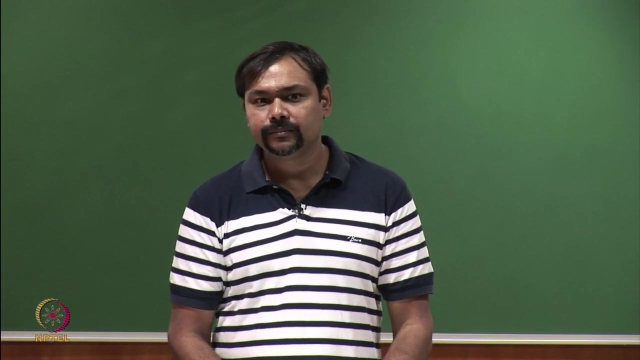 you have opened the battery or the voltage source. But if you short circuit the terminals of the battery, then a very large current flows through the wire which is shorting the battery. If the voltage source is an ideal voltage source, then the current which is flowing during this short circuit will be enormously. high It will be ideally infinite. practically it will be very high. So we cannot short circuit a voltage source because the current will be enormously high, or we do not know what is the exact magnitude of the current, only limited by the internal impedance of the voltage. 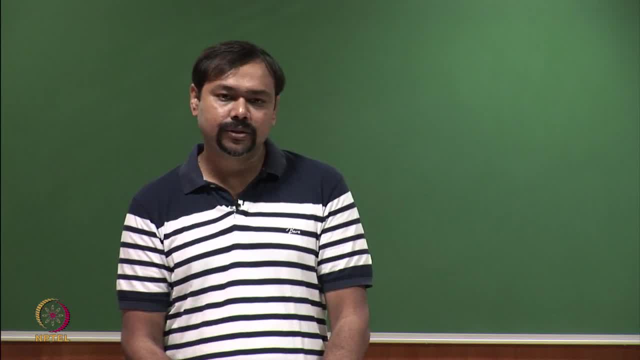 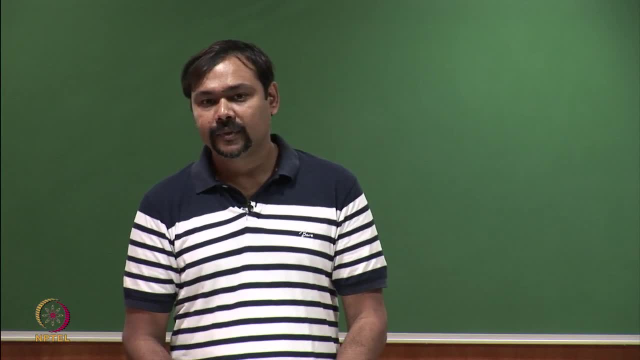 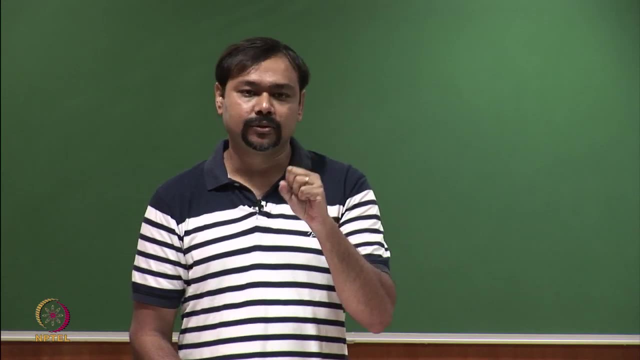 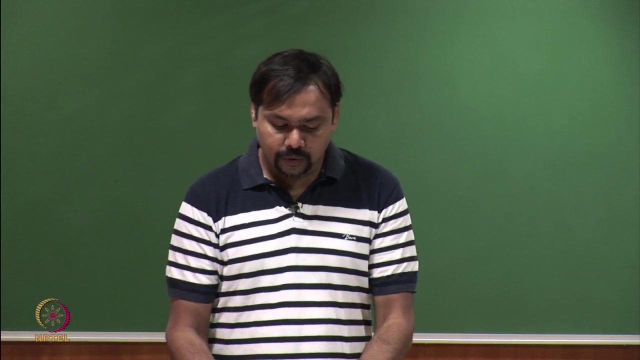 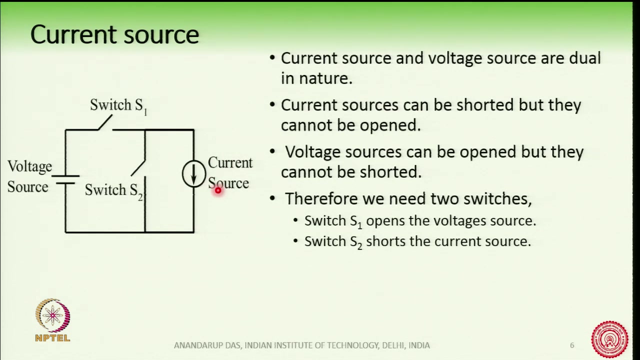 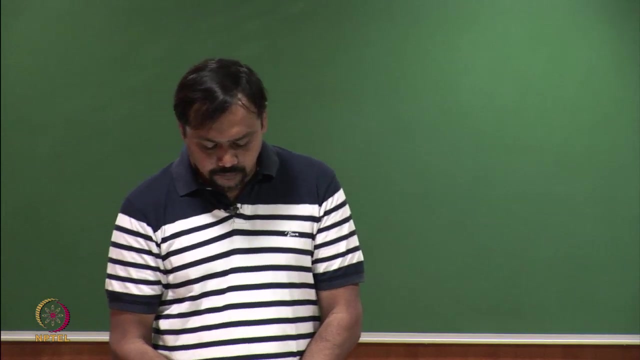 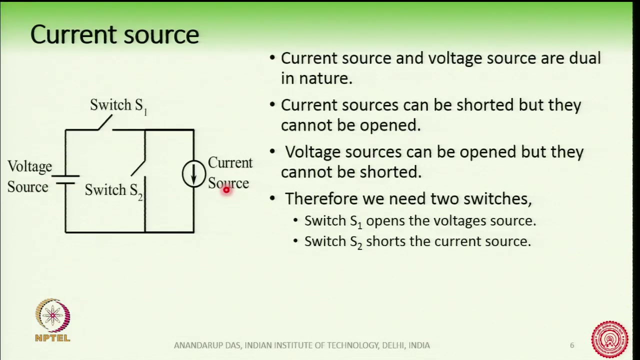 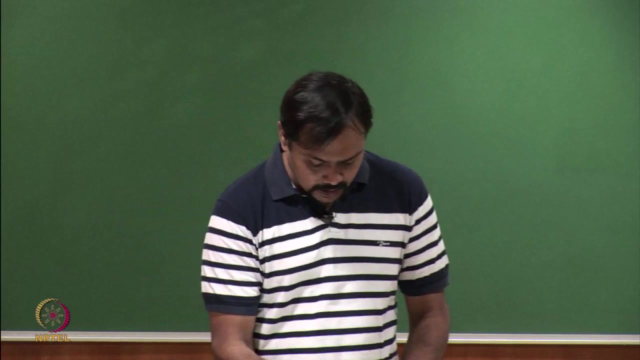 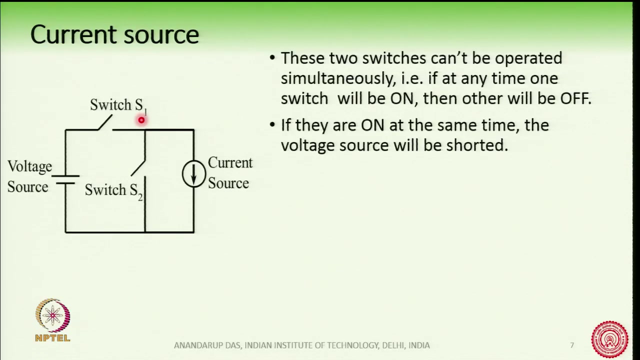 source. I turn on both S 1 and S 2 together at the same time, then I am going to short circuit the voltage source, which is not allowable. In a similar way, I cannot open both these switches together at the same time. In that case, I will open the current source, which. 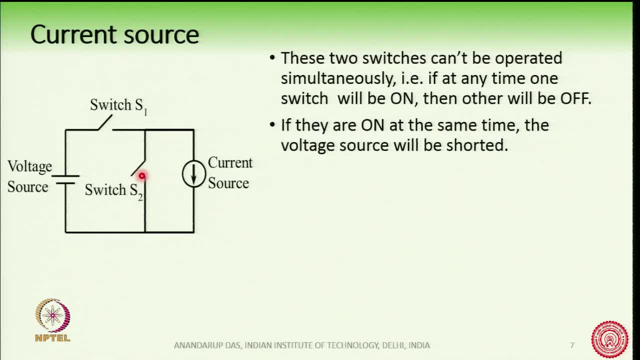 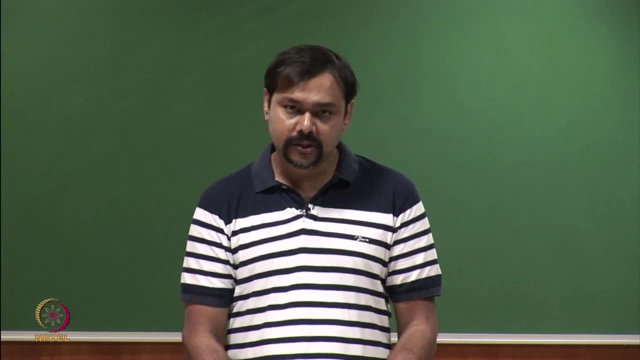 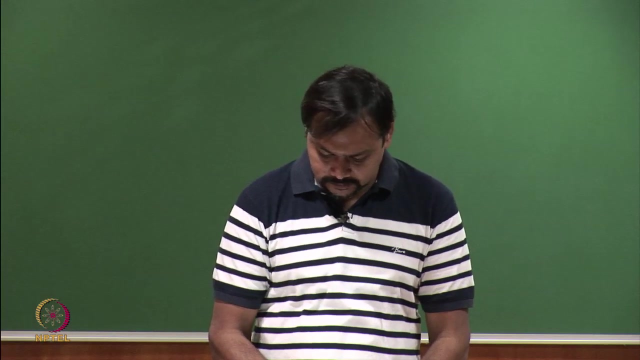 is again not allowed. So therefore, these two switches, S 1 and S 2, must be operated in a complementary fashion, Like when S 1 is on, S 2 is off, when S 2 is on, S 1 is off, like that. So they must be operated in the complementary fashion. 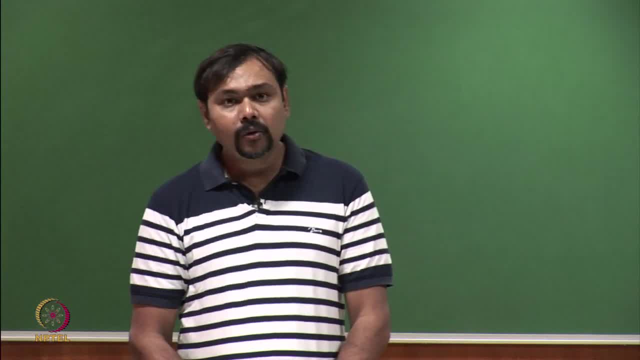 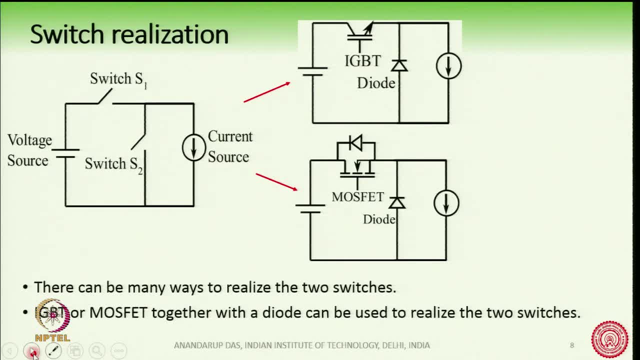 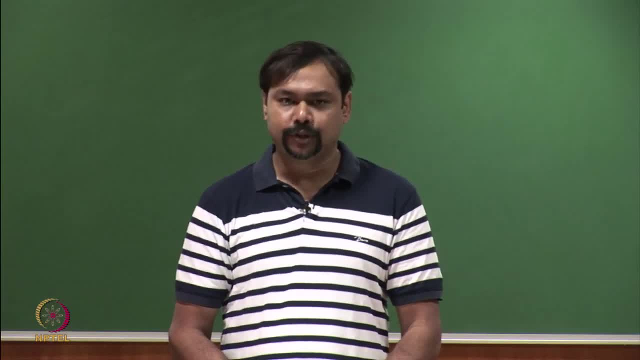 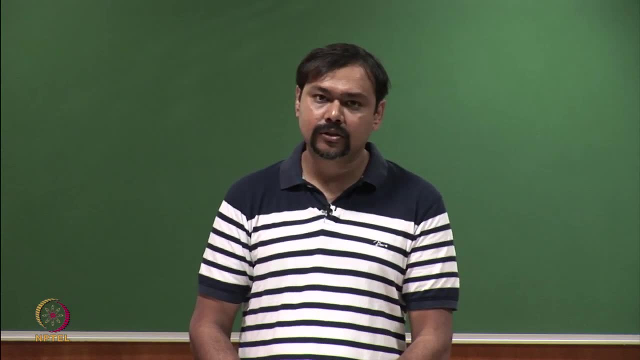 line every circuit, For example for short circuit, the cutoff process of x component. There are many ways to realize these two switches. One way is to use, for example, IGBTs or MOSFETs along with diodes. This is one of the simplest way of realizing these switches, For example: 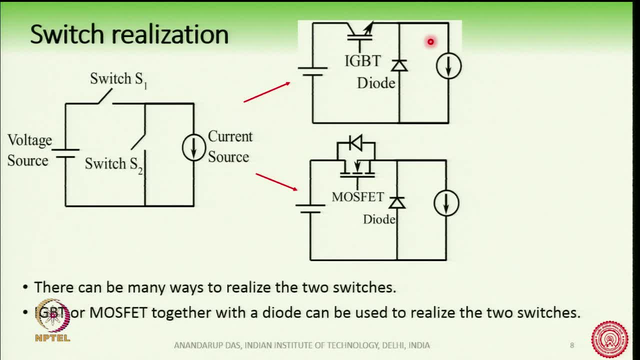 you can see on this one. on this circuit we have realized using IGBT and diode. Switch S 1 here is replaced by an IGBT. switch S 2 is replaced by the diode. In this lower circuit you can see: switch S 1 is replaced by the MOSFET. switch S 2 is replaced by the 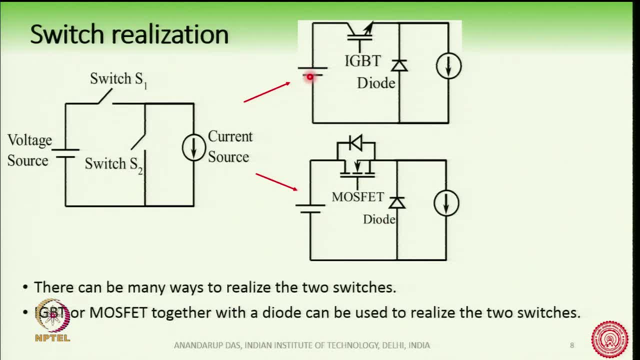 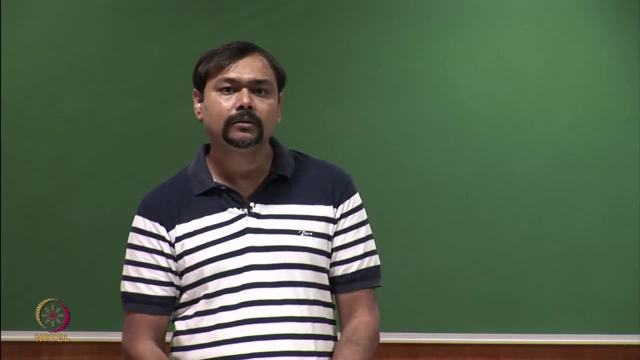 diode And we have the voltage source on the left and the current source on the left, And the current source on the right and the current source on the right. This is one way of realizing this circuit, using IGBT or MOSFET. 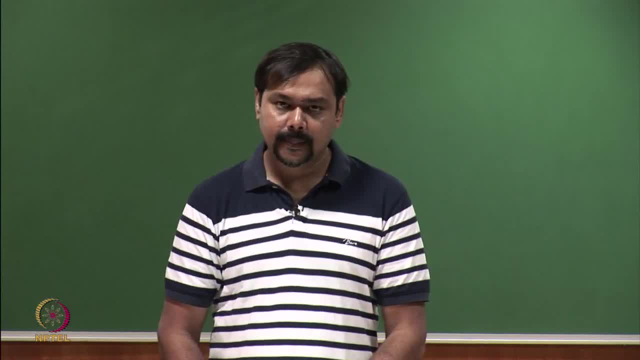 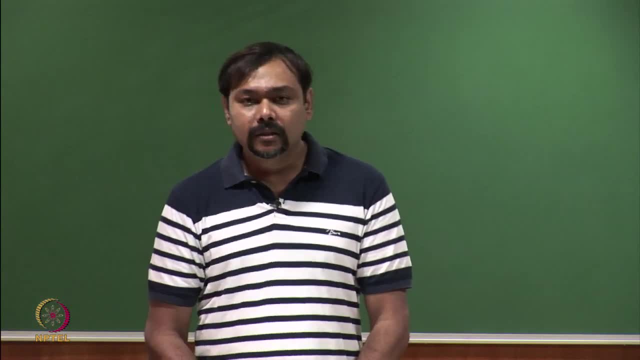 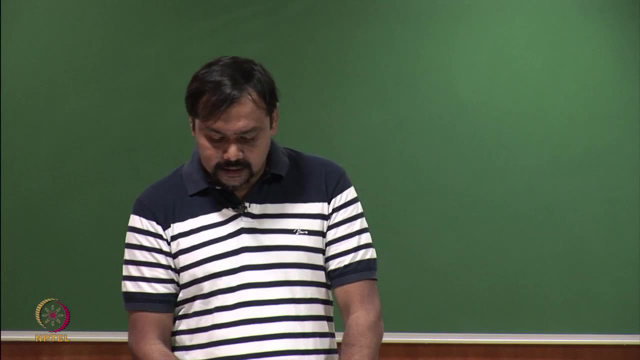 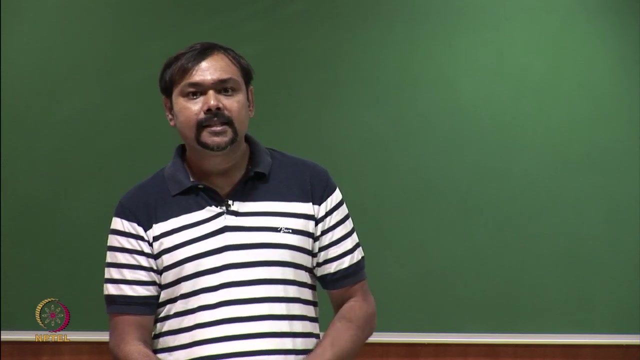 We can also use other types of switches. For example, thyristors can be used. However, in this course we will not talk much about thyristors. The reason is many past decades thyristors have been quite popular, But seeing the future, 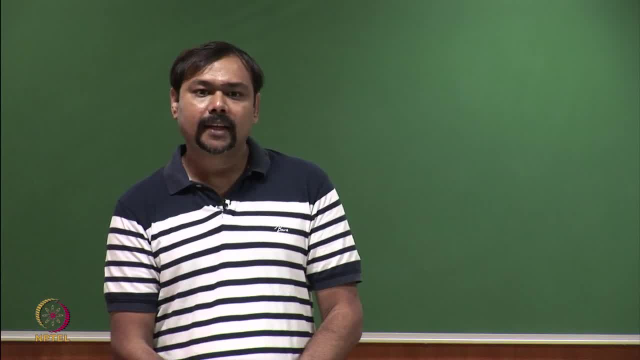 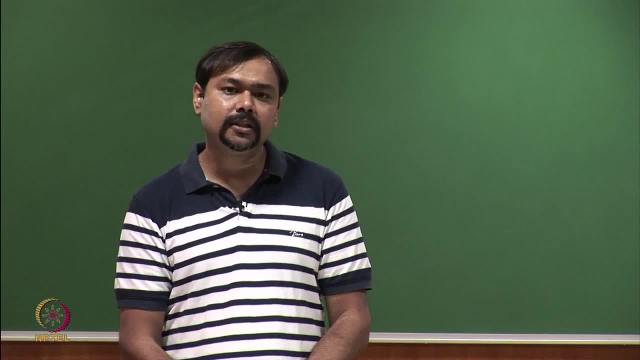 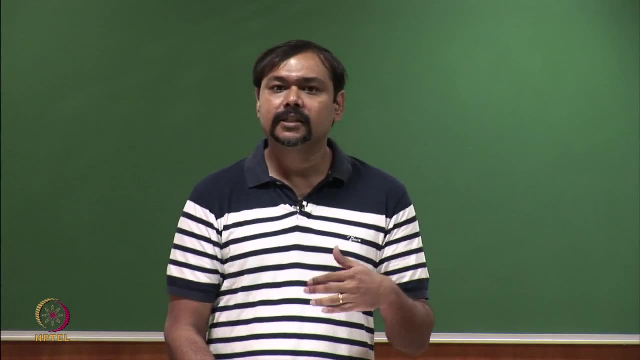 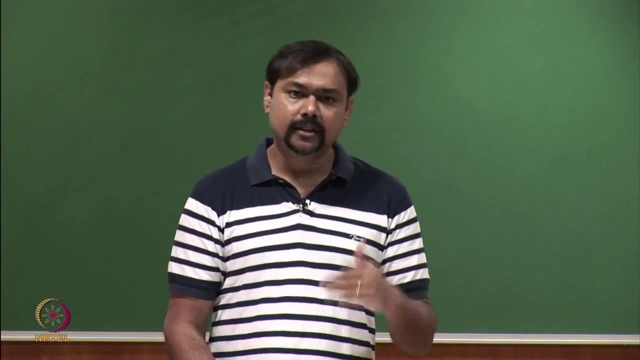 we see that in many of the applications, thyristors are going to be replaced, or have been replaced, with IGBTs or MOSFETs, Because one of the reasons is thyristors can be turned on and it is a semi controlled device. It can be turned on, but it cannot be turned off. The 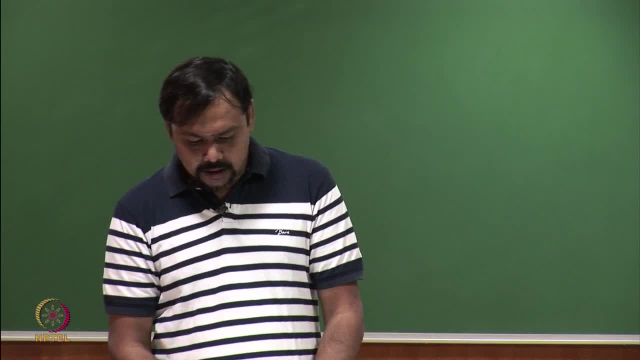 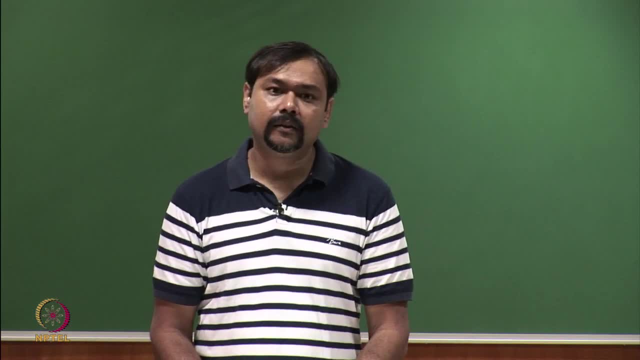 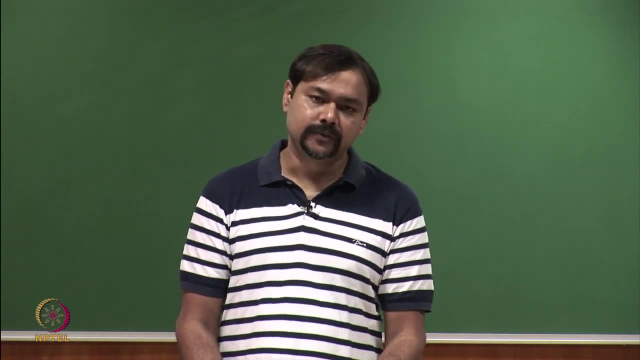 circuit decides how to turn it off. So we see that thyristors are going to be replaced mostly with IGBTs at the medium voltage level, and at the low voltage level MOSFETs will be predominant. That is what we see in near future, say for at least 10 to 15 years. So 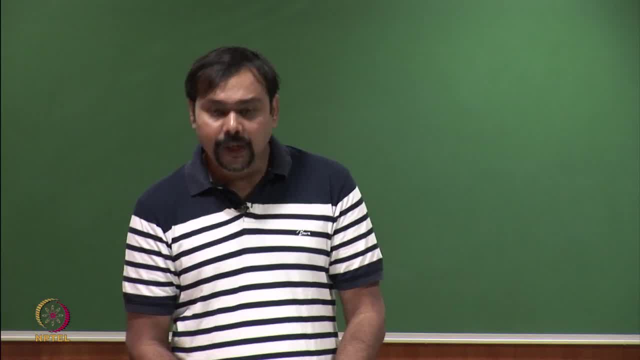 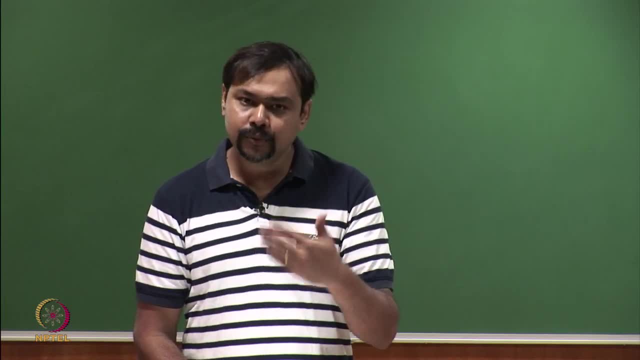 being 15 to 15 years from now, So we are not going to talk about thyristors much in this course. Of course, thyristors will be used at very high power levels. LCC based HVDC, for example, will still continue. 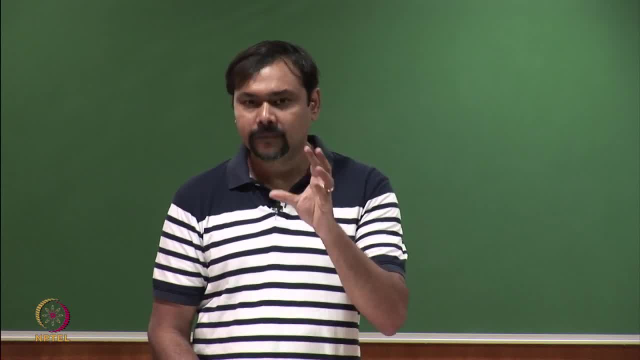 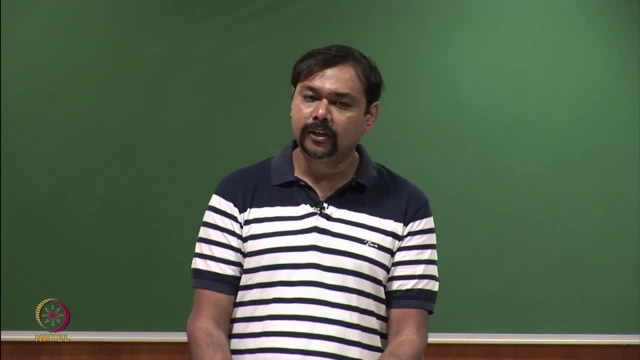 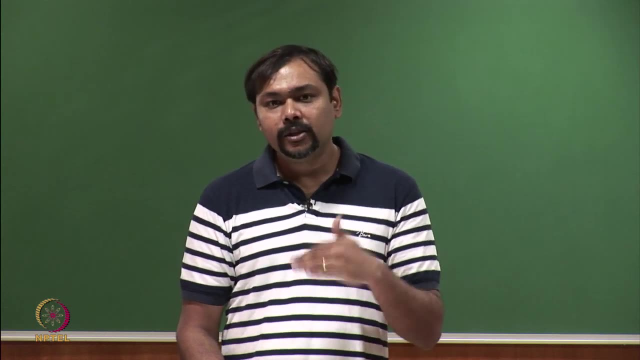 to use thyristors. But they are very specific applications and in many new developments that is going to that is going on here now In the field of high power, high voltage, HVDC, for example, power electronics, The thyristor, newer developments are all happening with IGBTs. 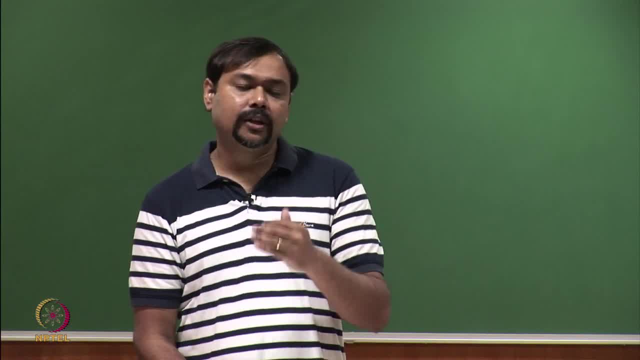 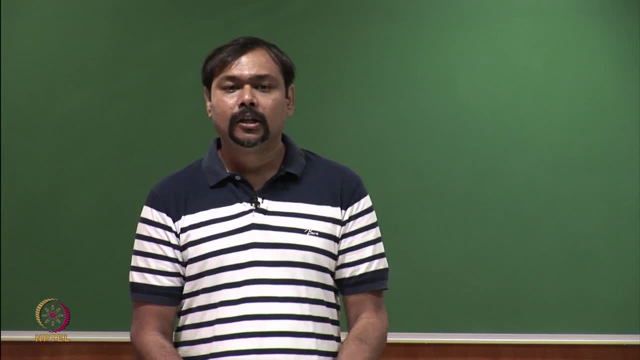 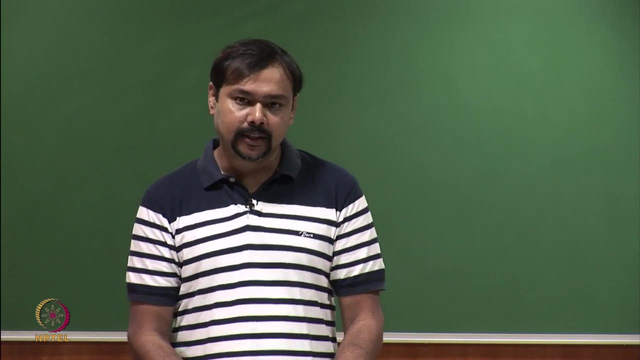 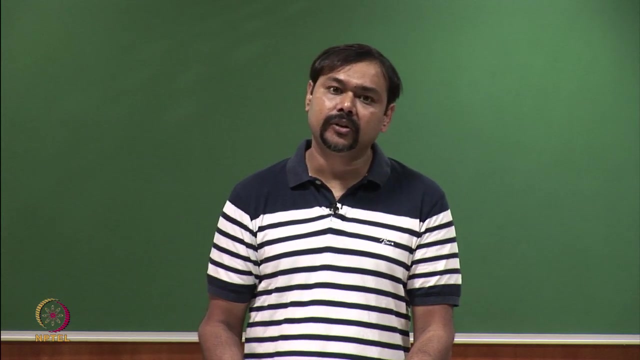 So, and in particular we can also say that with wide band gap devices coming at least at the lower voltage levels, huge presence of wide band gap devices are expected in near future. So we will not talk much about thyristors in this course and mostly concentrate on IGBTs. 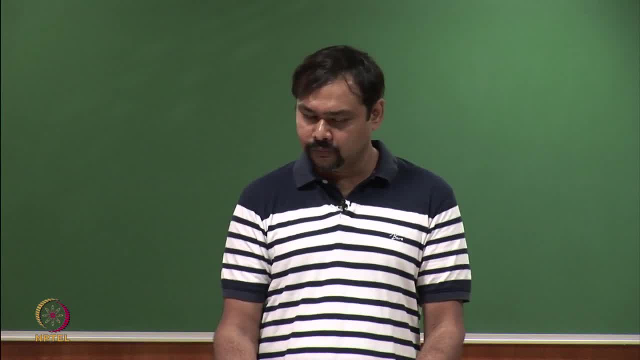 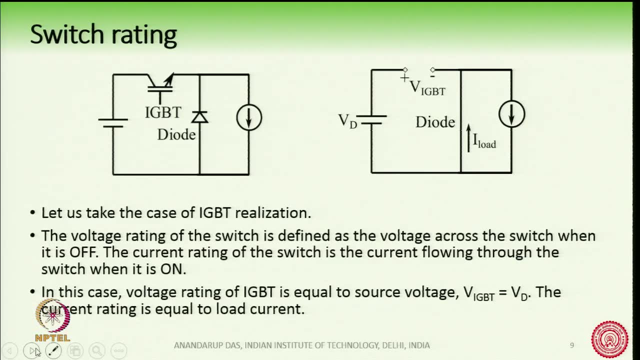 at the medium voltage level and sometimes MOSFET at the low voltage level. So let us take the case of this converter with an IGBT based realization, which I have shown in this circuit. here We have a voltage source, We have the current 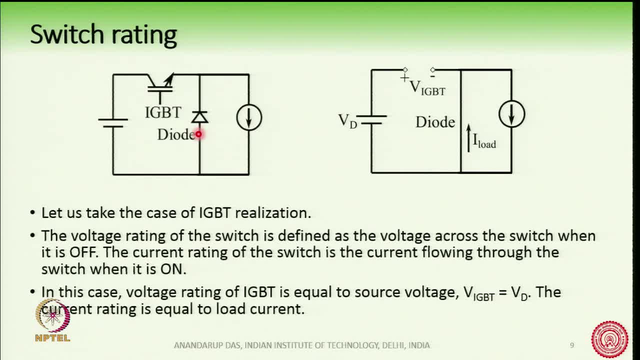 We have the current, We have the current source, the IGBT and the diode here. Now, what is a switch rating? Switch rating is the rating of the switch that we are going to use. There are two. there are many ratings of the switch, which you can see from the data sheet. of a switch. but there are two very important rating of a switch. One is the voltage rating and one is the current rating. What is a voltage rating of a switch? The voltage rating of the switch is defined as the voltage across the switch when it is. 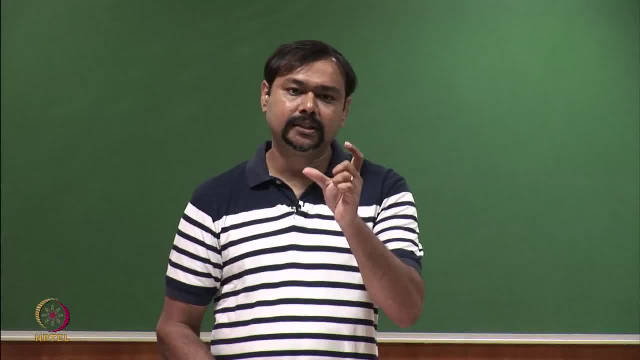 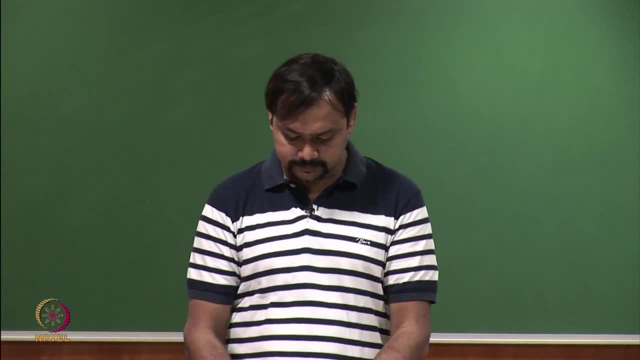 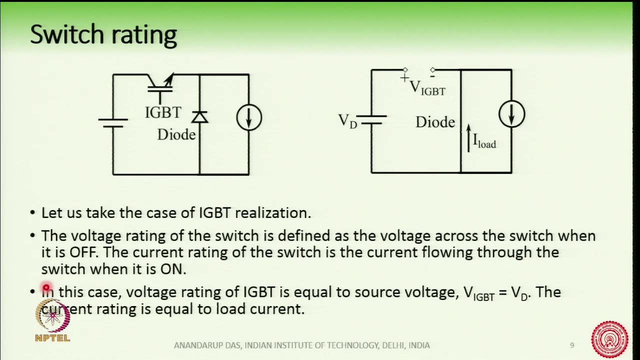 off. So when the switch is off, how much voltage is impressed across the switch? that determines the voltage rating of the switch. What is the current rating of the switch? The current rating of the switch is the current flowing through the switch when it is turned. 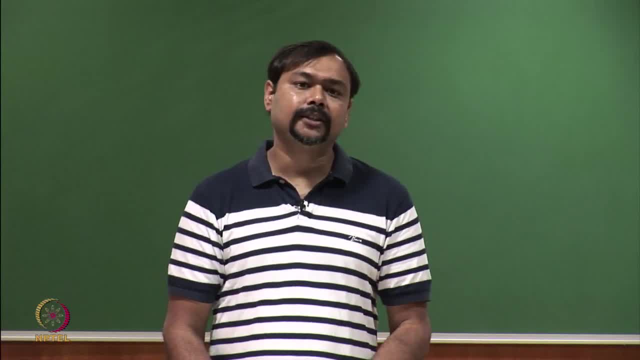 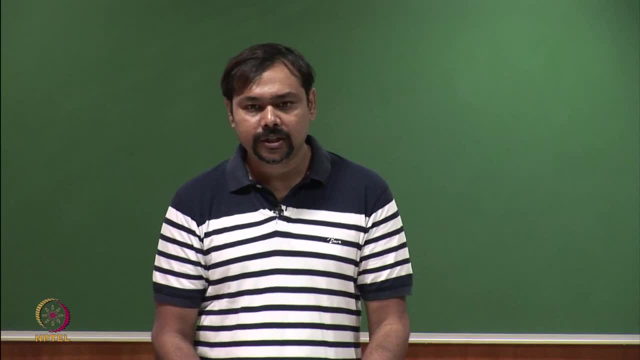 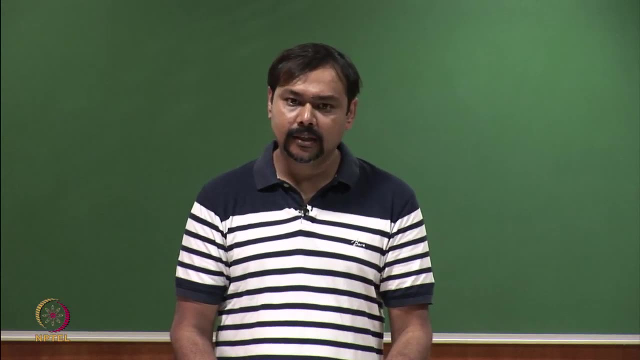 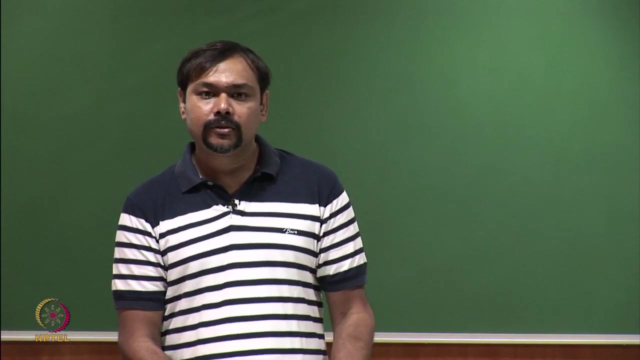 on. There are many other ratings of the switch switch, for example temperature rating of the switch, and then there is also transient rating of the switch. Many other rating of the switch is present which, if you open the data sheet of any device, you can see the different ratings of the switch. but these two rating 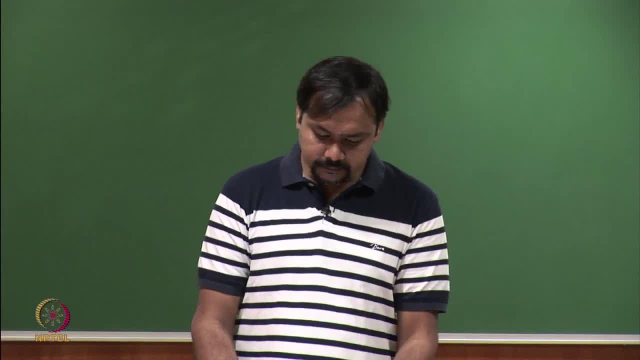 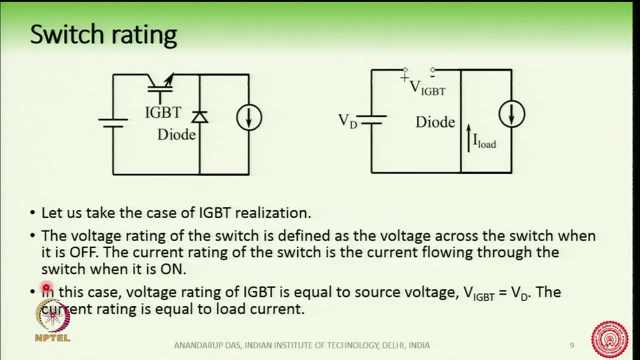 are very important: voltage and current rating of the switch. So let us try to find out first what is the voltage and current rating of the IGBT and diode in this particular circuit. So when we suppose we want to find out the voltage, 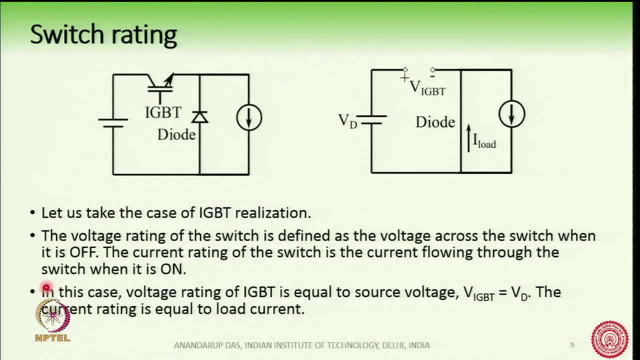 rating of IGBT. So, in order to find out the voltage rating of IGBT, we see, or we try to find out, what is the voltage across IGBT, The IGBT when it is turned off. So when it is turned off, the circuit, when the IGBT. 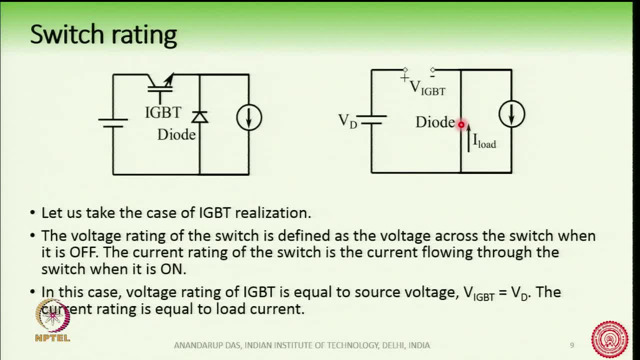 is turned off, the circuit looks like this: As I have told earlier that S 1 and S 2 are complementary in nature, So if the IGBT is turned off, the diode is turned on. So I have put a short circuit here and through this short circuit the load current is flowing. 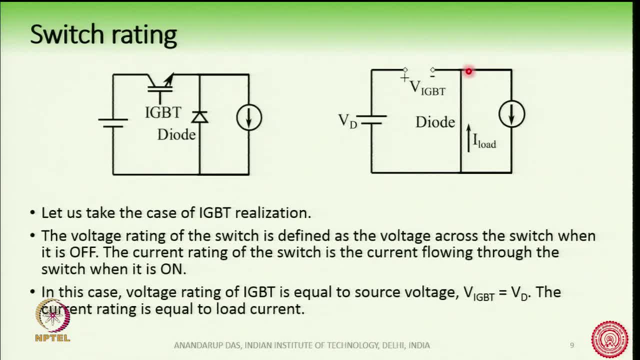 Since the IGBT the diode is short circuited, therefore the negative terminal of this source is connected here, while the positive terminal is connected here, And so we can see that the voltage across IGBT during this time is equal to the source voltage. So this 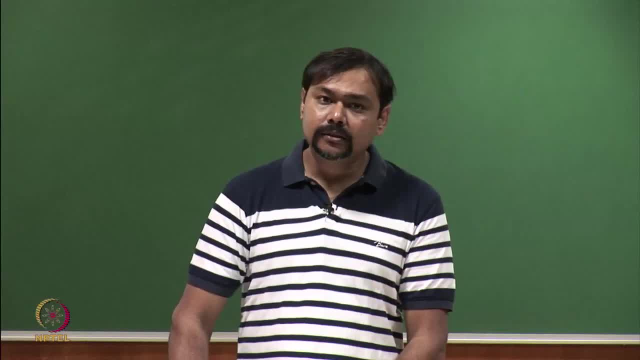 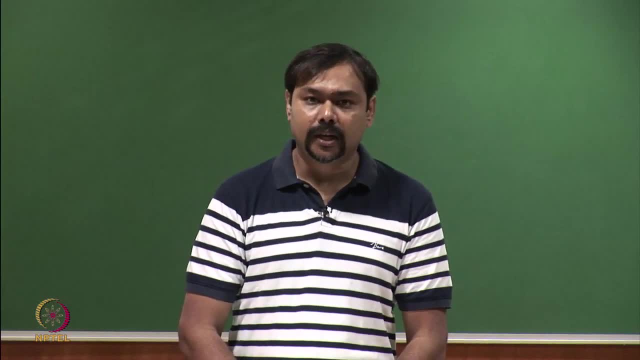 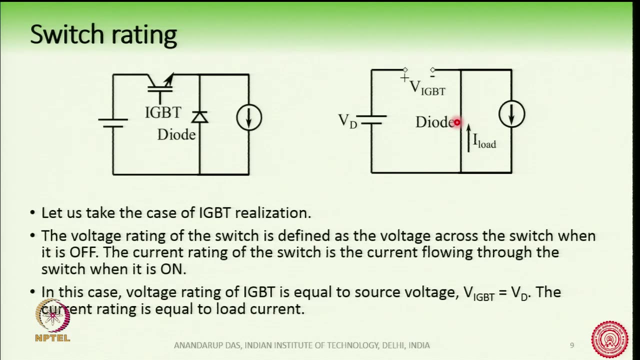 is the IGBT. Now, what is the current rating of the IGBT? The current rating of the IGBT will be equal to the load current, because when the IGBT is conducting, the diode will be turned off because it will be reverse, biased, And so the current of the load current is flowing through the IGBT and therefore the IGBT is turned off. The current rating of the IGBT is equal to the load current, So the voltage rating of the IGBT is equal to the source voltage and the current rating of the IGBT. 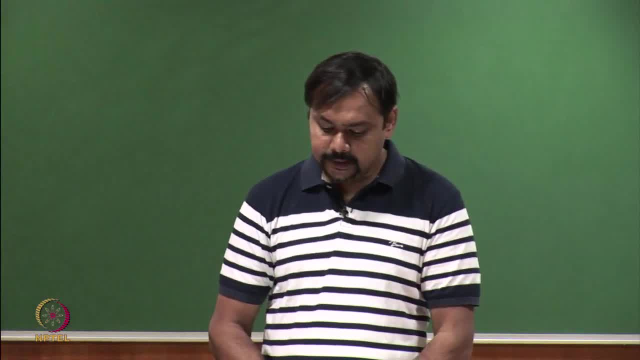 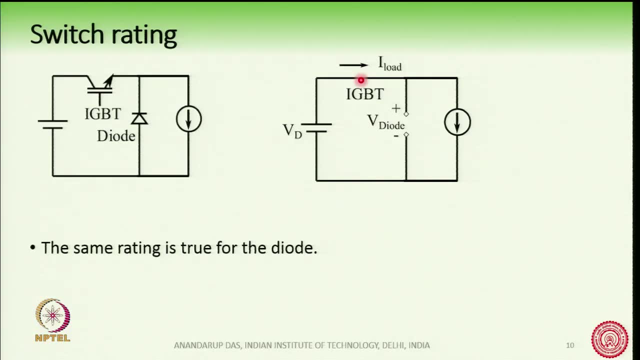 is equal to the load current. What about the diode? Again, for the diode, we see that when the IGBT is turned on, then the diode is turned off. And since the diode is turned off When the IGBT is turned on, So this terminal, positive terminal, comes here and the negative 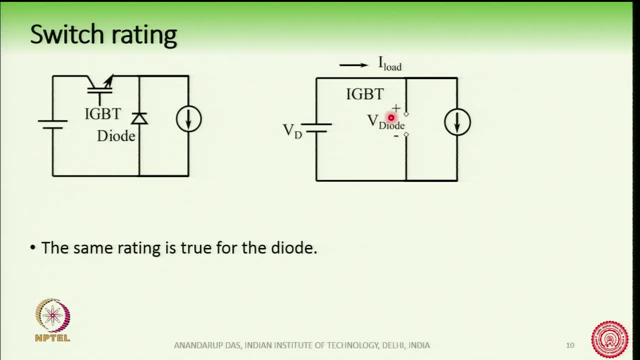 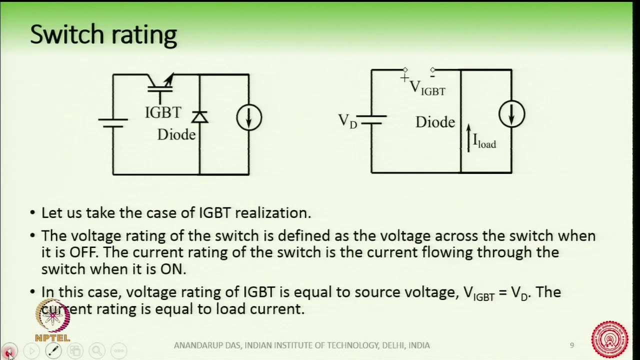 terminal is here. So the voltage across the diode is equal to the source voltage. So, therefore, voltage rating of the diode is equal to the source voltage. And what is the current rating of the diode? The current rating of the diode- I have already shown it here- is: 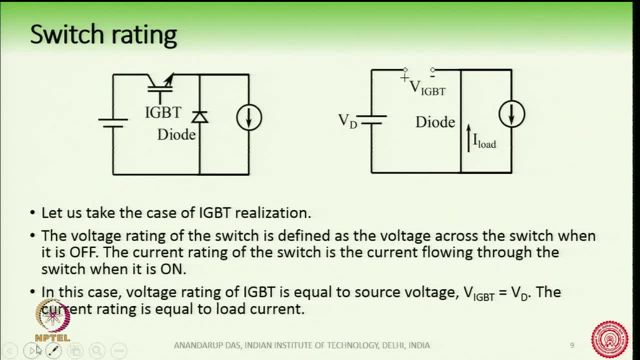 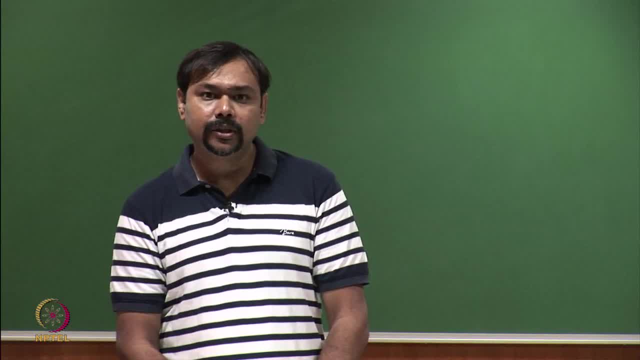 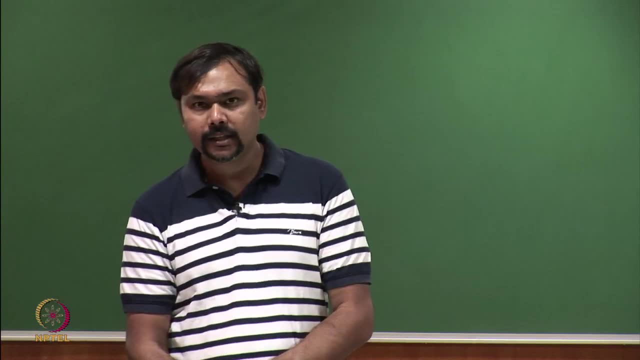 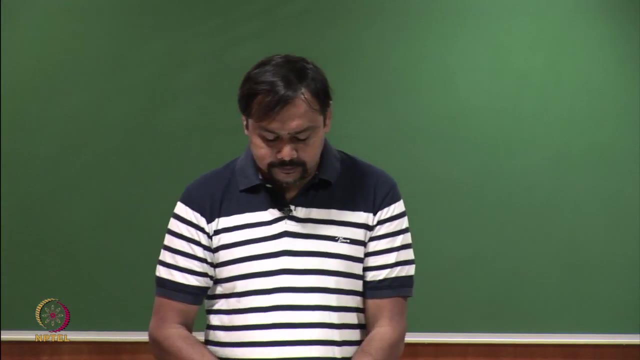 equal to the load current. So therefore the voltage and current rating of both the IGBT and the diode is are same. Voltage rating is the source voltage and current rating is the load current. Now the circuit which we have so far developed is this: 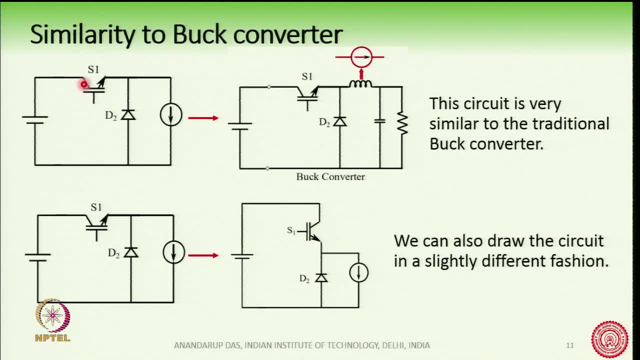 The circuit which we have so far developed is this. This circuit which we have so far developed is this one with the switch diode and the voltage and current source. Those who are a little bit familiar with power electronics will immediately see a similarity of this circuit with a Buck converter I have drawn. 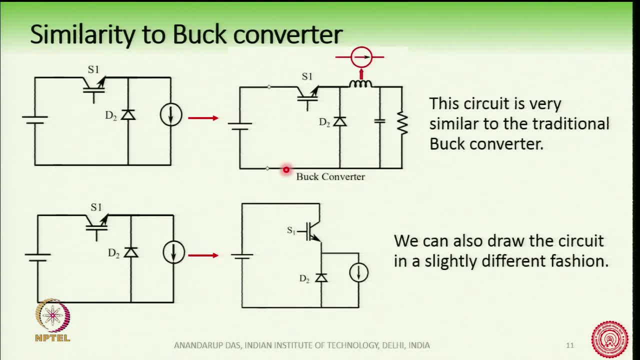 a Buck converter here. Ok, And the Buck converter here is the current rating of the diode. So this circuit is equal, And the buck converter also has voltage source. and then there is a load. there are two switches here. there is an inductor and a capacitor. 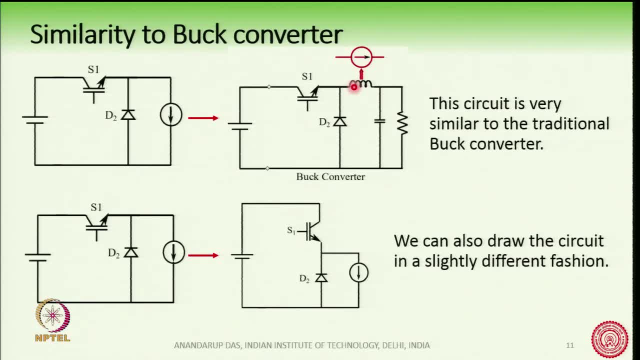 If we consider the current flowing through the inductor as a current source, then we see that the buck converter here has very much similarity with the circuit that we have developed so far. So I can also redraw this circuit. whatever I have drawn, I can draw it a little bit differently. 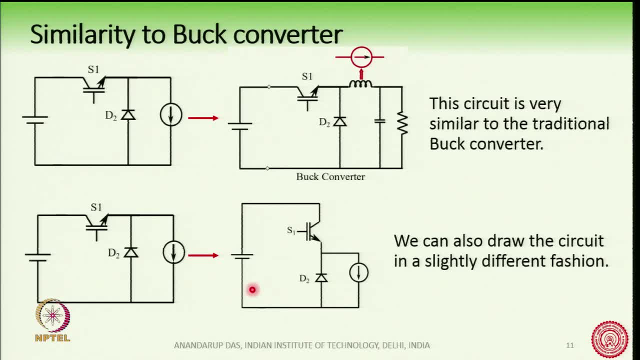 the same circuit, but I have drawn it a slightly different, as I am showing it here in this circuit. Ok, So I have placed the switch in a vertical position and the diode here at the bottom and the current source. like this: This circuit is exactly similar to the left hand circuit. 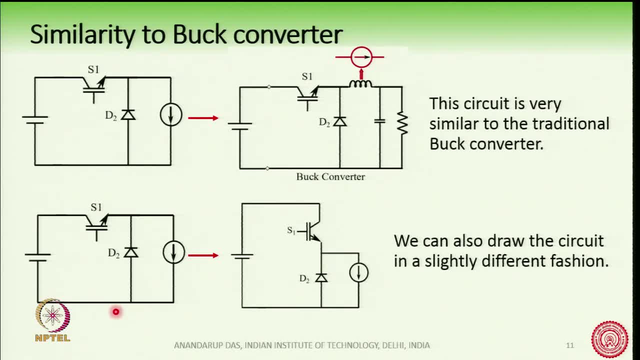 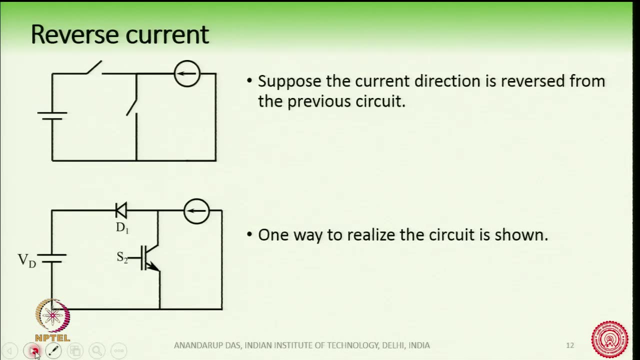 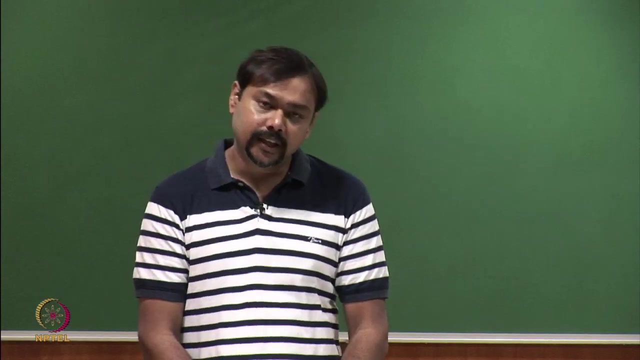 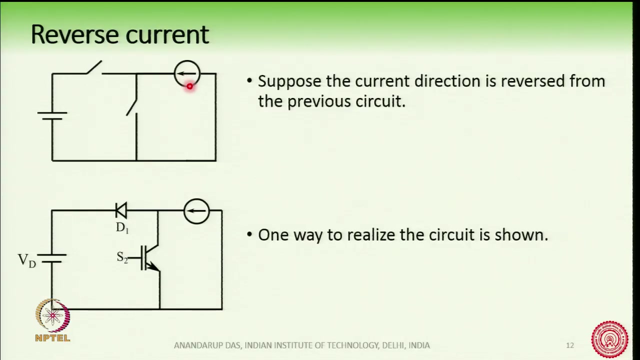 So both these circuits are same. I have just redrawn it. I will come to. I will come back to this circuit a little bit later. Now, suppose I have now changed the direction of the current. So now here, let us assume that we have changed the current direction from right to left earlier. 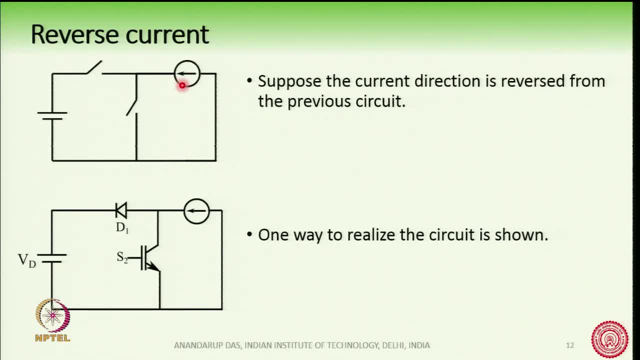 it was from left to right. Now I have changed the direction from right to left. What will happen now to the circuit? So how can I realize the circuit now? So what I can do, This is one way of realizing the circuit. 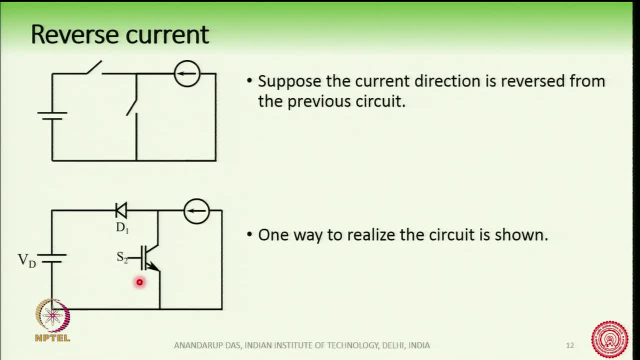 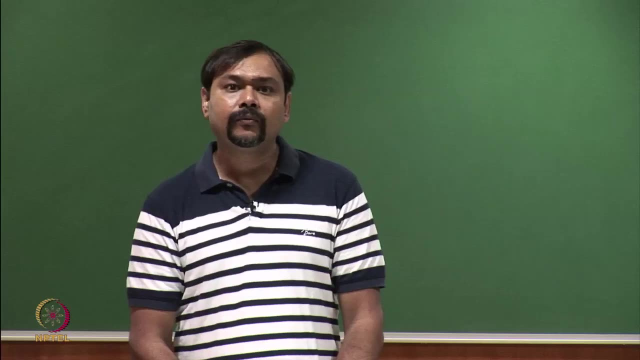 As you can see, here I have interchanged the positions of the diode and the transistor, So the IGBT has come down here and the diode has been moved here compared to the previous circuit. So this is one way of realizing a circuit with the voltage source here and the current. 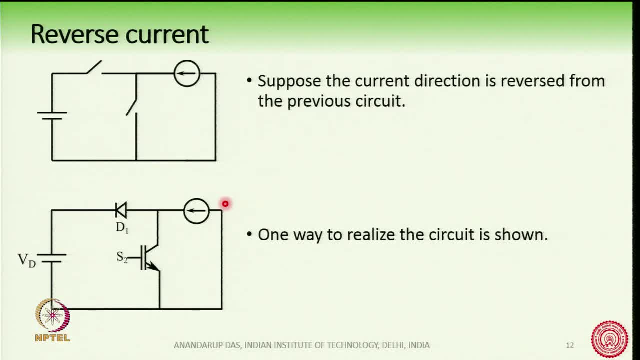 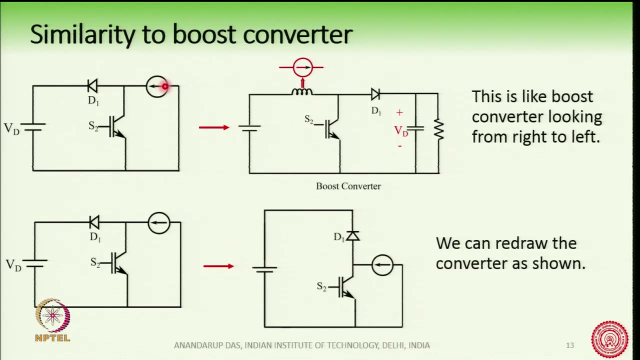 source here, where the current source, the current direction is from right to left. So this circuit, which is the current, where the current direction of is from right to left, is very similar to a boost converter, but you have to look from right to left. 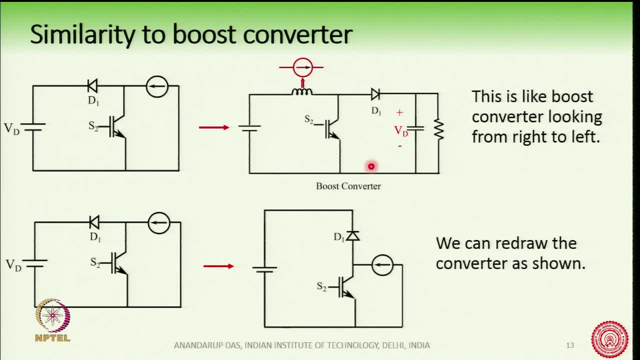 So, for example, this is a traditional boost converter and you have, this is the voltage source and this is the load here. In a boost converter we have an inductor at the front part of the circuit and then we have two switches here And then the capacitor which acts as a voltage source. 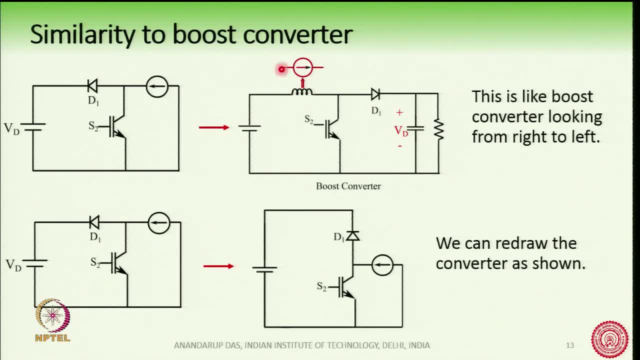 So if we replace this inductor with a current source like this, then we see that, looking from left to right, looking from in this direction, from left to right, we see that there is a current source and there is a switch, control switch, and there is a diode here and then. 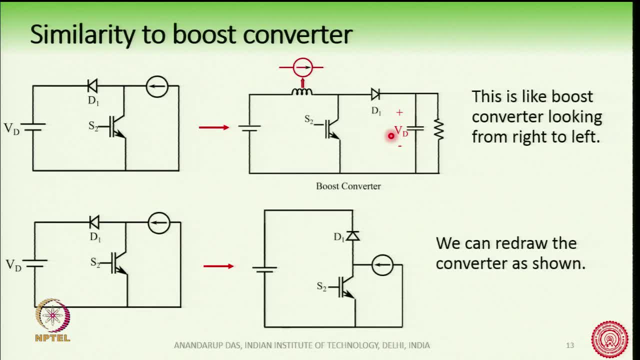 there is a voltage source. Similarly, looking from on this circuit, if you look at in this circuit and see that there is a current source here, there is a switch here, there is a diode here and there is a voltage source here. So for this circuit, looking from right to left, and for this boost converter, looking 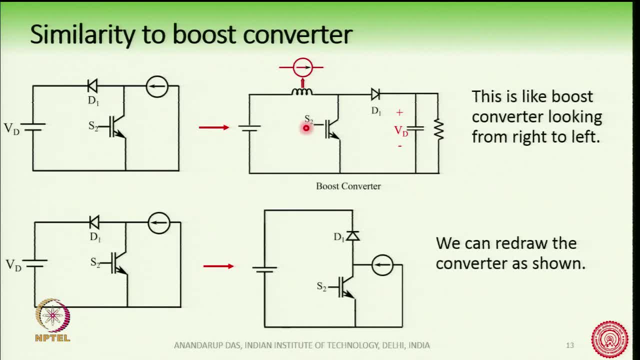 from left to right, we see that these two circuits are very, very similar. Looking from left to right, there is a current source, switch diode and a voltage source. Looking from right to left: current source, two switches and a voltage source here. So they are very similar. 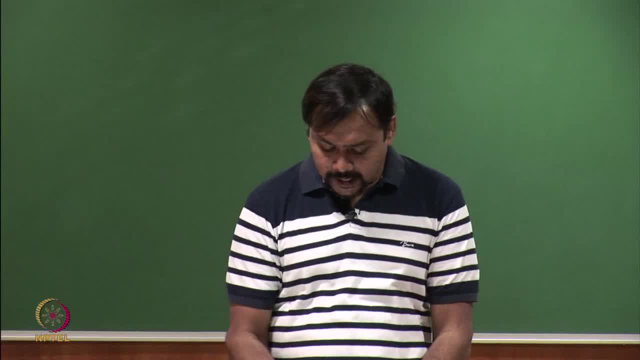 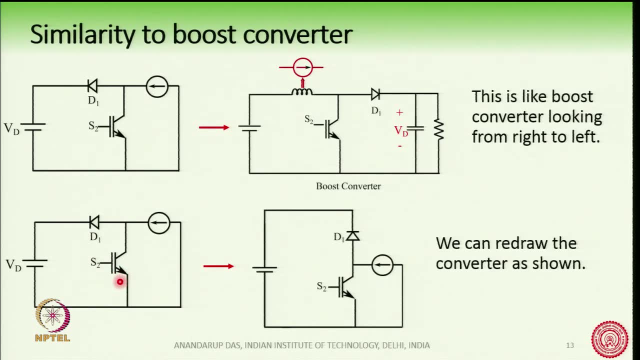 Again. Therefore, what I will do now, I will again redraw this circuit in a slightly different fashion, as I have shown it here. You can see: the voltage source is here and the voltage source is here. The current source is here and the current source is here. 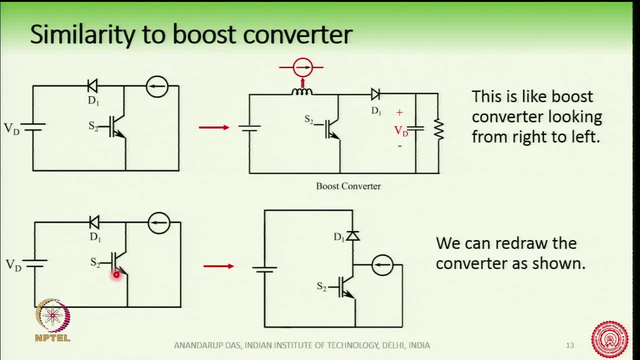 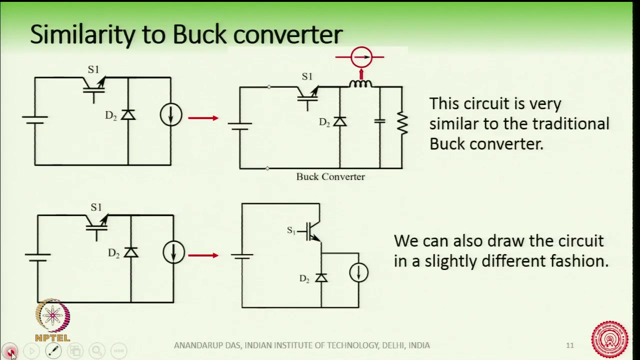 The switch, the transistor here, S 2 has been now put down here And the diode there has been redrawn in a slightly different fashion here. So we have now redrawn the circuit, Now combining this circuit which was derived from the buck converter. 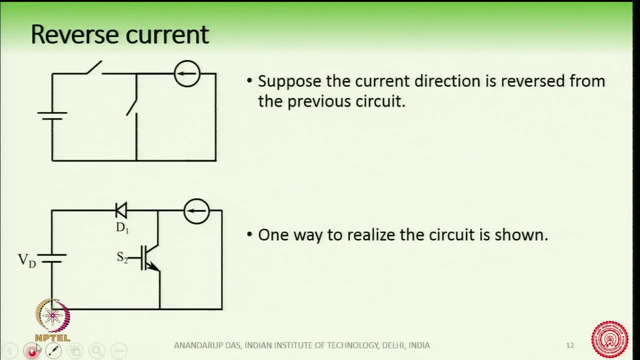 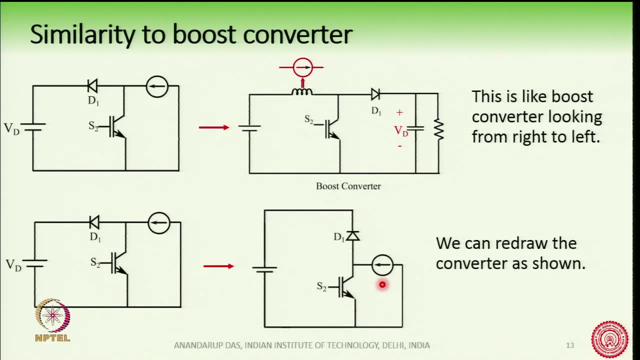 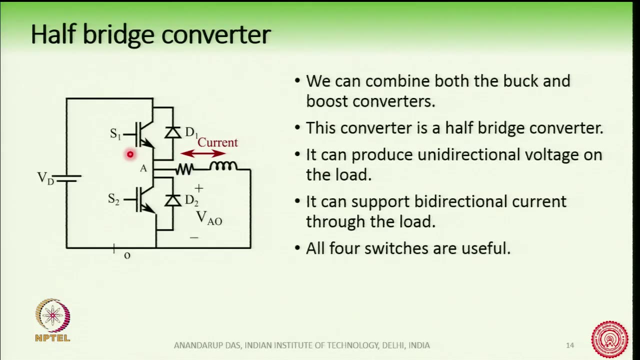 And the circuit which was derived from the boost converter analogy. we can combine these two circuits and how does it look? It looks like this: This is the current source. here is the current source present, which is shown by an R L load here: 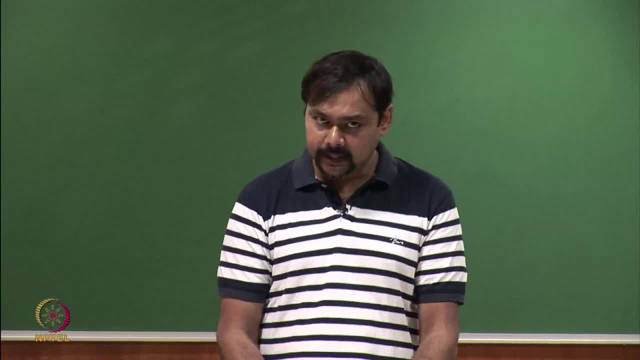 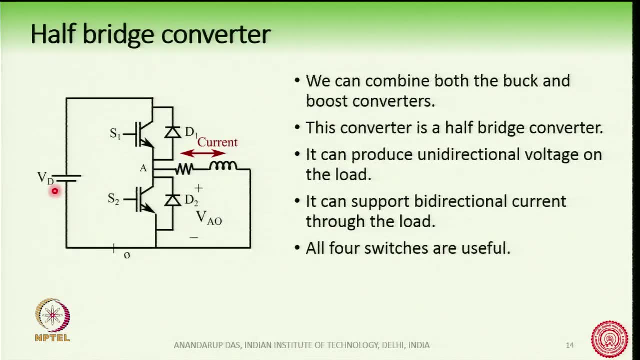 The current source is bidirectional in nature, So it can be positive or negative. This is the voltage source here, And then we have two transistors or two IGBTs here and two diodes here. 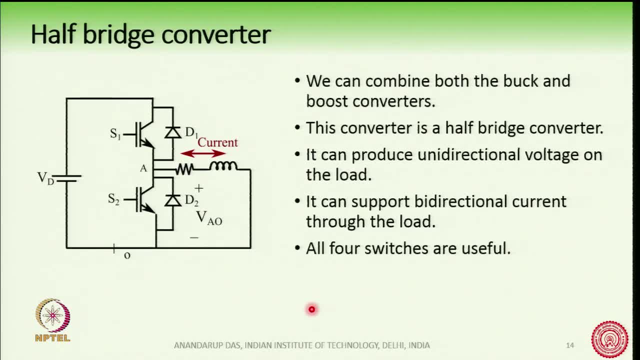 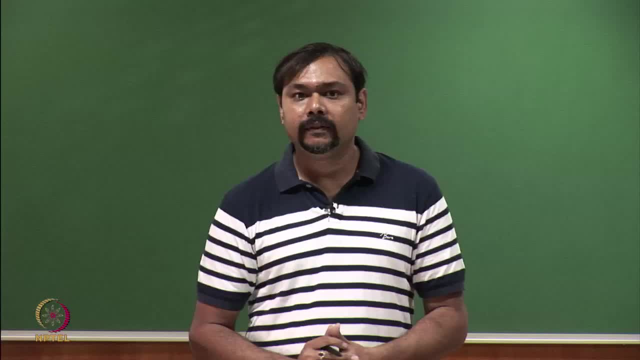 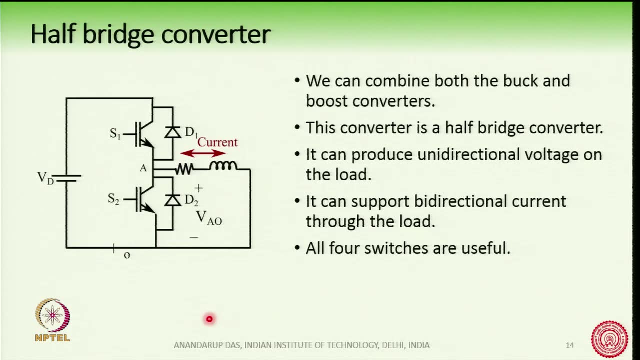 Also from the buck converter and boost converter topologies, the analogy. from that analogy we can combine this buck and boost converter with a single circuit like this, And this circuit is called the half bridge converter. The half bridge converter is one of the basic topologies. 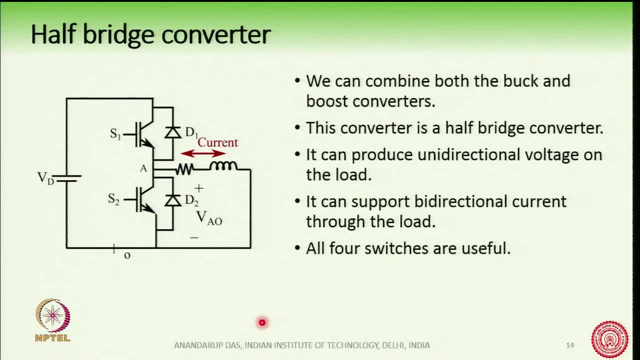 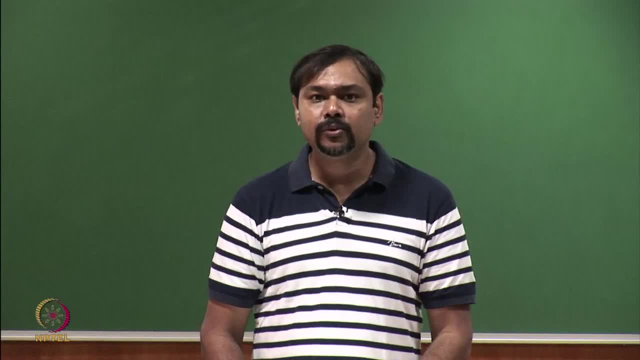 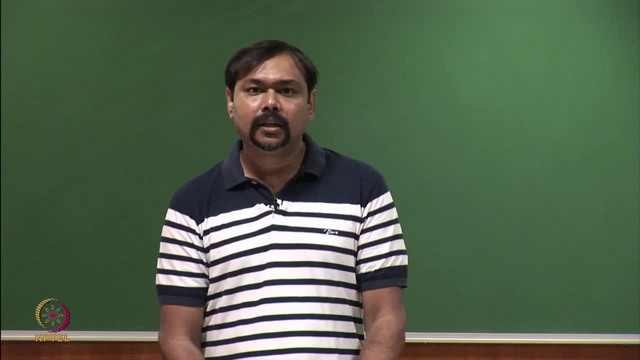 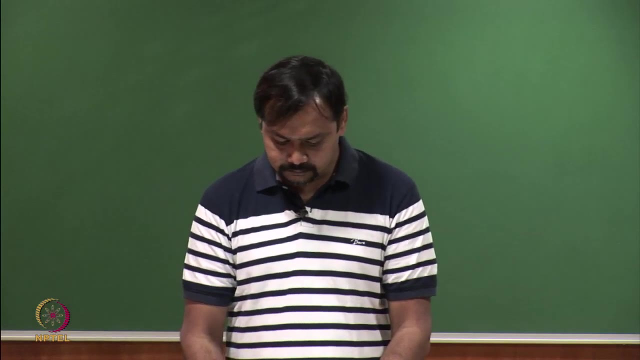 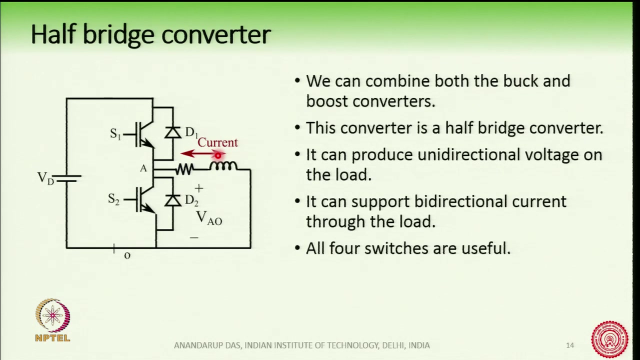 of power electronics And also for this course. half bridge converter is something which will be used frequently and derivations of half bridge. So understanding the half bridge converter is very important for this course. So we see that in this half bridge circuit the voltage here at point A can be controlled by the switches S 1 and S 2.. If you measure, 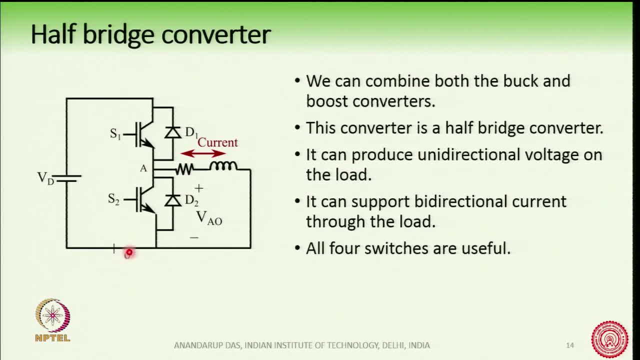 the voltage at point A With respect to point O at the bottom. then we see that the voltage at point A can be either 0 or V? d. So when the lower switch is on, then the voltage is 0 between A and